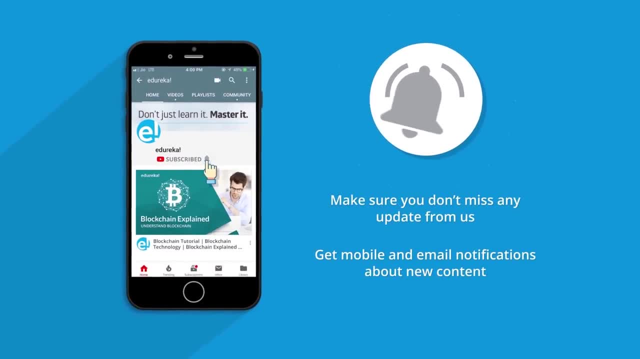 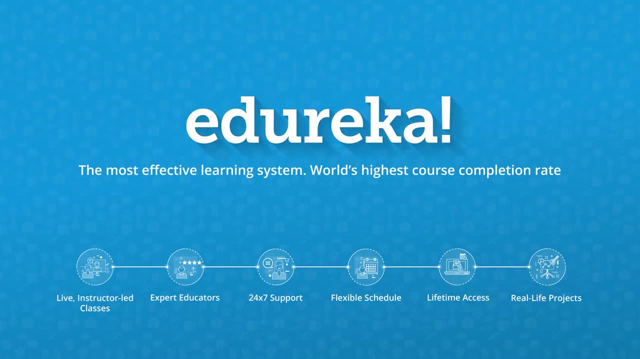 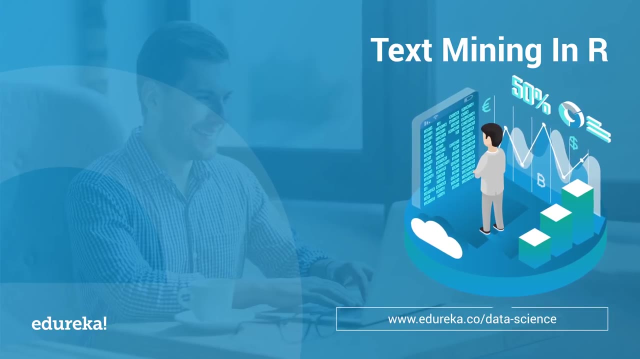 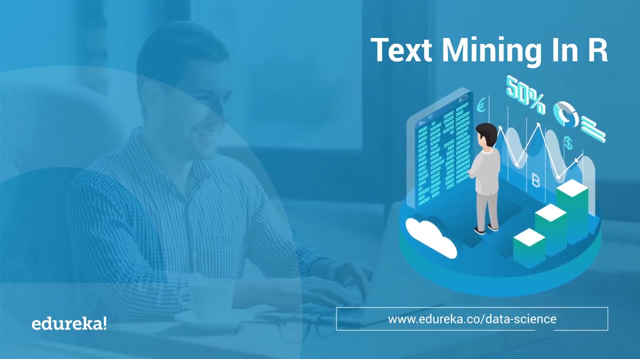 Hi everyone. this is Zulekha from Edureka. With the increasing importance of text analysis in communication, research, text mining and natural language processing are becoming extremely important. With this in mind, let's begin our today's session. We'll mainly be focusing 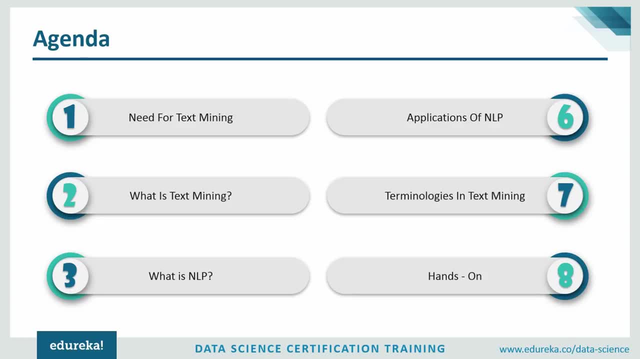 on the various methodologies used in text mining in order to retrieve useful information from data. Alright, so let's move ahead and take a look at today's agenda. We're going to begin the session by understanding the importance of text mining. Next we'll see. 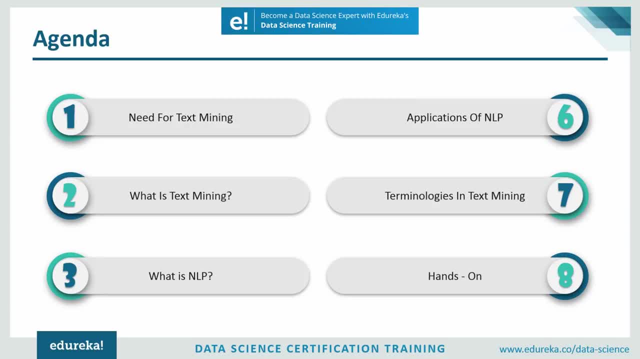 what exactly text mining is and where it is used. After that we'll move on and look at what exactly NLP, or natural language processing, is, And here we'll also discuss the relation between text mining and NLP. After that we'll move ahead and discuss a few applications. 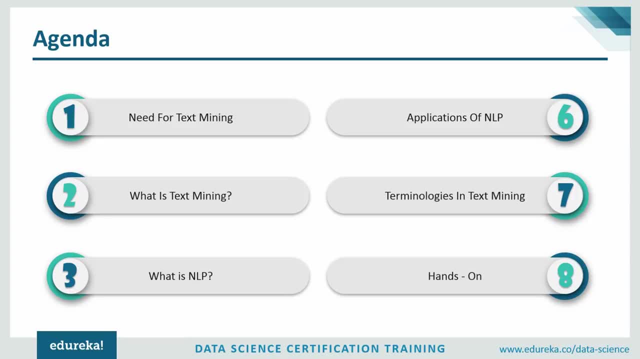 of NLP. We'll talk about the various domains that NLP is used in. Once we're done with that, we'll go through important terminologies used in text mining, such as stemming, tokenization, document term matrix, stop words and so on. Finally, we'll end the session with a detailed 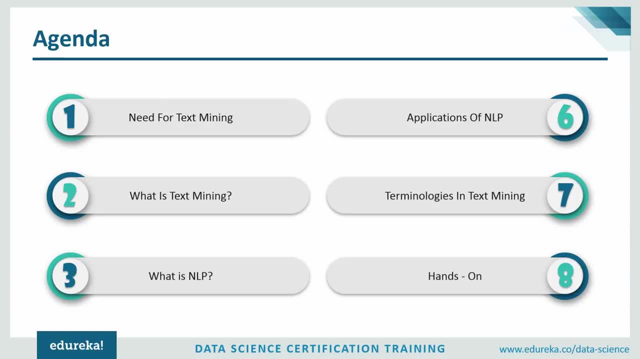 demo where we'll use a set of documents and perform various text mining methodologies. in order to understand the text mining process Without wasting any further time, let's move ahead and take a look at our first topic. Okay, so the need for text mining. So, guys, let me tell you that the amount of data we 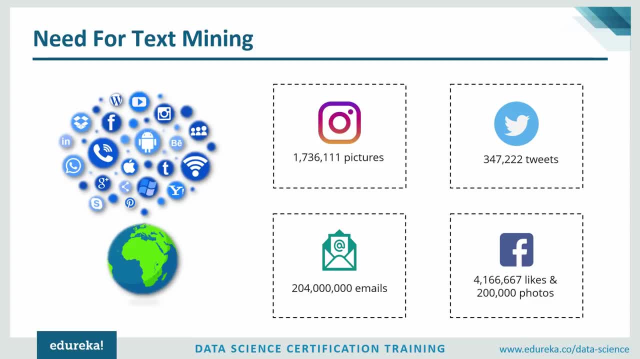 produce every day is truly astonishing. Okay, so we produce around 2.5 quintillion bytes of data every single day, And this number is only going to increase. Okay, so, with the evolution of communication via social media, we generate tons and tons of data. So, guys, 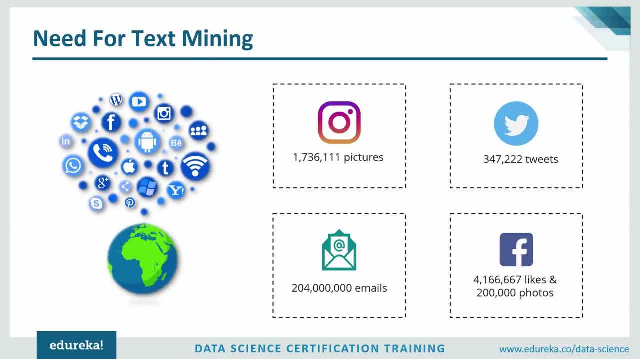 the numbers are on your screen. According to a recent survey, around 1.7 million pictures are posted every minute on Instagram. Similarly, we have around 347,000 tweets on Twitter every minute and around 204 million emails go out every single. 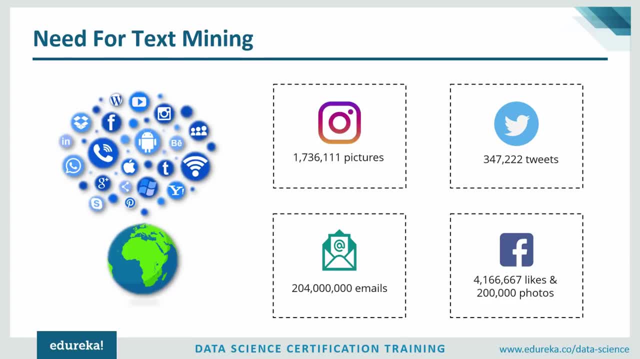 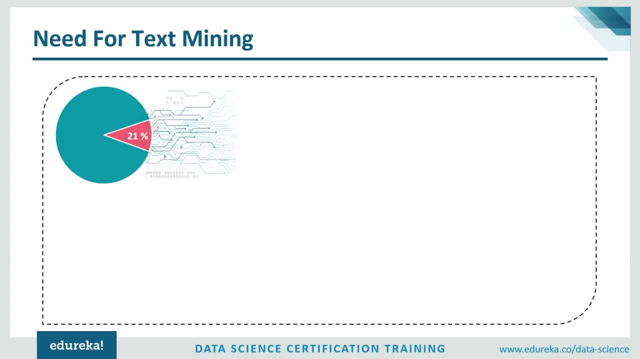 minute. So you guys can imagine how much of data we're producing through emails, through text messages, through pictures, through likes and comments, and all of that All right. Now, not only that, out of all the data that we generate, only 21% of the data that we generate, 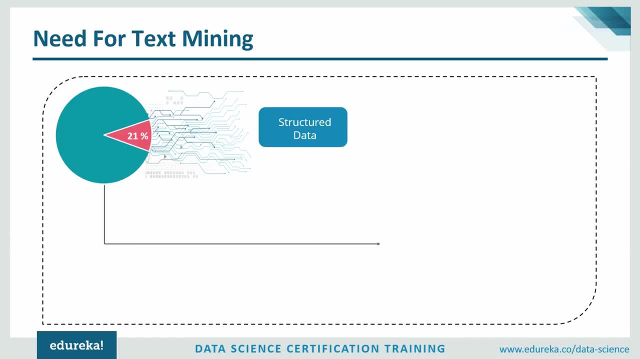 is structured and well-formatted. The remaining of the data is unstructured. The major sources of unstructured data include text messages from WhatsApp, Facebook likes, the comments on Instagram, the bulk emails that we sent out every day. All right, all of this accounts. 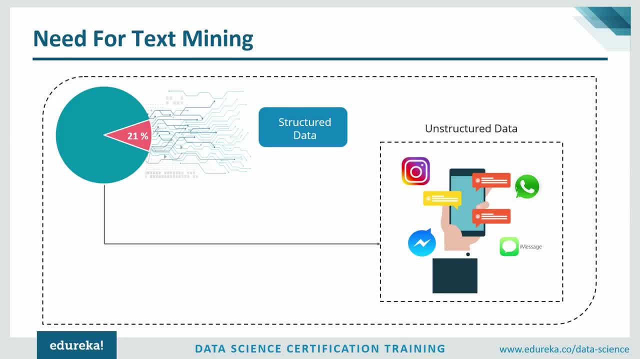 for the unstructured data that we have today. Now the question to ask here is what can be done with so much of data. The data we generate is used to grow businesses. By analyzing and mining the data, we can add more value to the data that we're producing. All right, 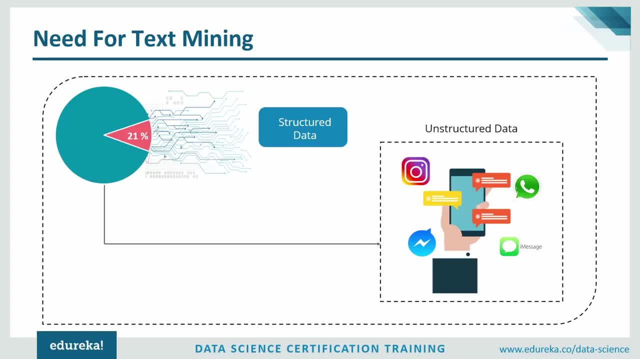 I hope that answers your question, So let me just close my talk first. So let me share to a business. this is exactly what text mining is all about. okay, text analytics or mining is the analysis of data available to us in a day-to-day written or spoken language. okay, it's amazing that. 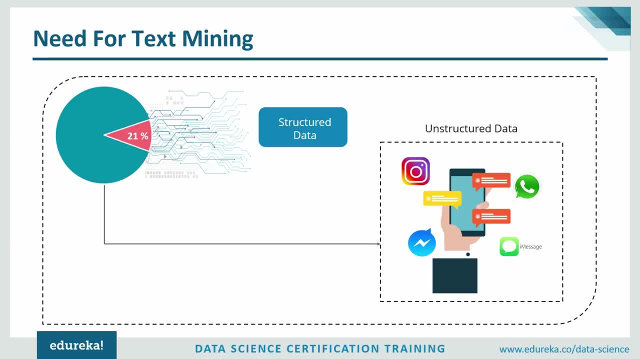 so much data that we generate can actually be used in text mining. okay, so all the word documents that we have, the powerpoint presentations, chat messages, emails- all of this is used to add value to a business. so, guys, data is always useful when you want to add value to a business. so, guys, data is. 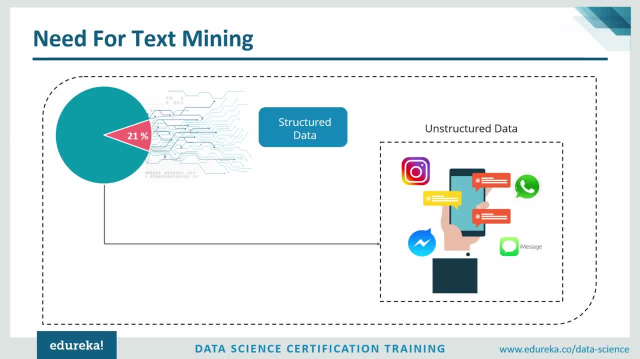 the key to every single business. if you know how to analyze your data correctly, if you know how to find hidden patterns from your data and retrieve good information from your data, your business is going to be successful. all right. the only reason why companies like netflix, amazon, walmart are 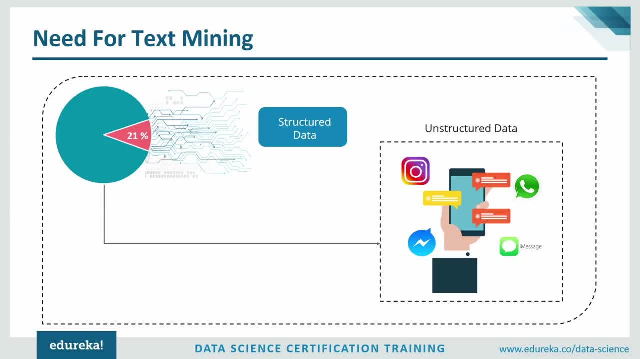 doing very well right now is because they have learned how to analyze their data correctly. okay, the only way to add value to your business is through extracting useful information from all the data that you get. okay, this data can be from your customers, it can be through social media, it can be these tweets, it can be likes. so, with all of 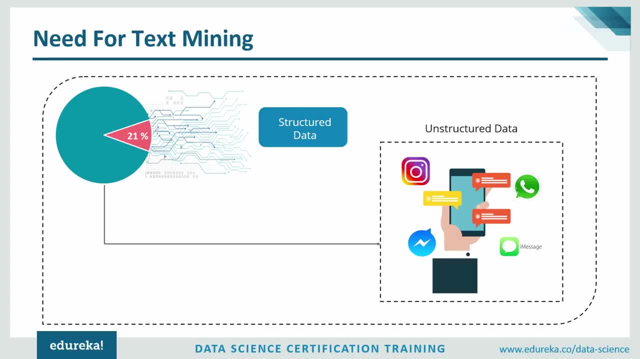 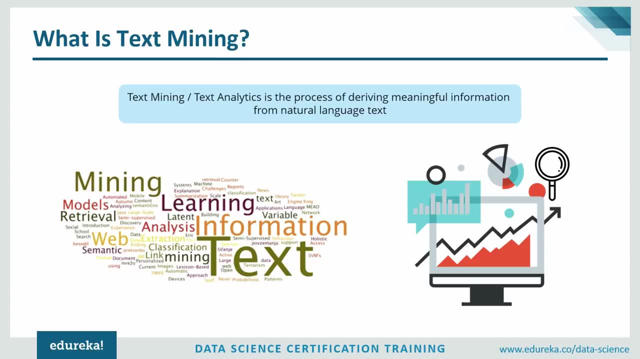 this information, you can actually grow your business. all right, and this is exactly why we need text mining. now let's move ahead and look at what exactly text mining is. so, guys, text mining, or text analysis, is the process of deriving meaningful information from natural language text. so all the 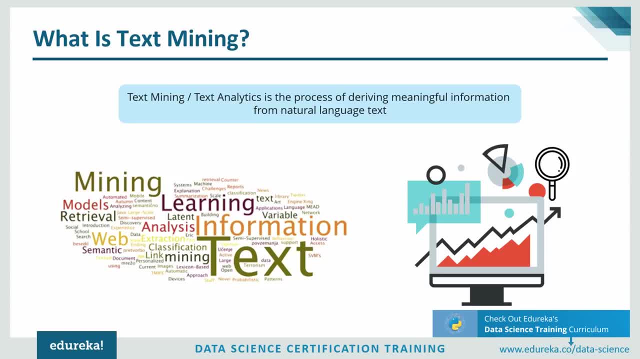 data that we generate through text messages, emails, documents and files are written in natural language text, correct, and we are going to use text mining to draw useful insights or patterns from such kind of data. okay, now let's take a look at few examples that show how we use text mining every 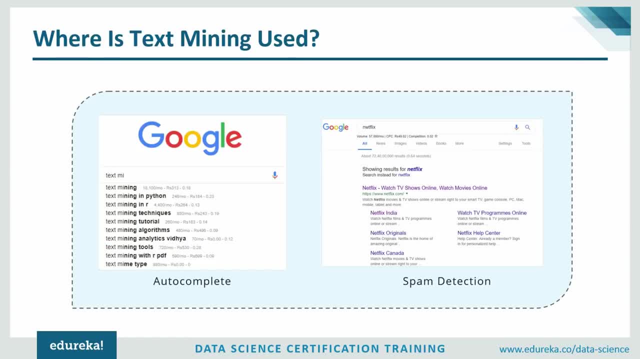 single day, okay. so, guys, we all spend a lot of time surfing the web. now, have you ever noticed that if you start typing a word on google, you immediately get suggestions like these, right? so if i start to type text mining, i immediately get a text mining- text mining in python or text mining in r: this: 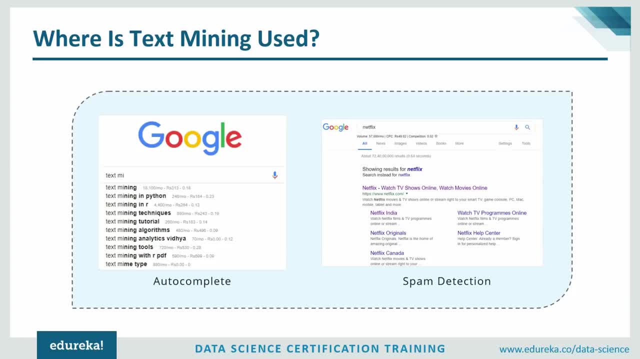 feature is also called autocomplete. all right, it will basically suggest the rest of the word for you. okay. similarly, we also have something known as spam detection. okay, so over here is an example of how google recognizes the misspelling netflix, all right, and it shows results for keywords that. 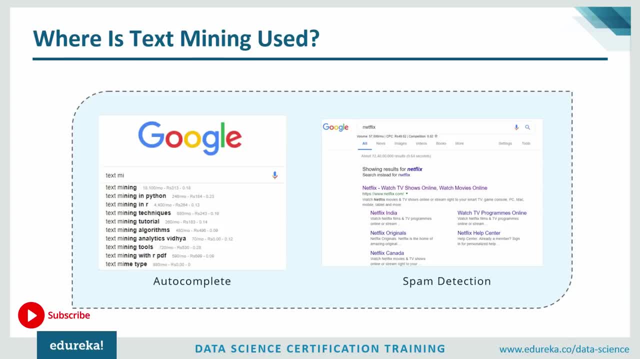 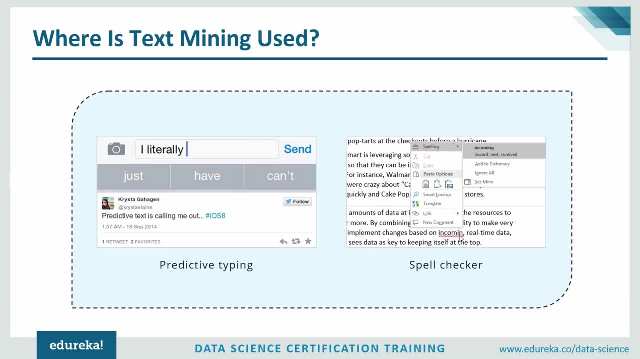 match your misspelling. okay, so the spam detection is also based on the concept of text mining, and all right. next, we have predictive typing and spell checkers. features like autocorrect email classification are also applications of text mining and nlp- all right. so, guys, predictive typing is 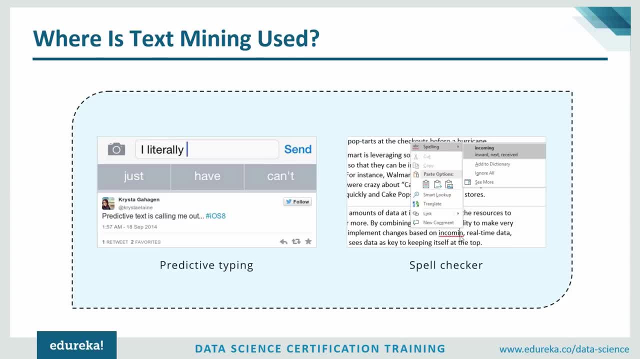 pretty understandable. it just predicts what you might type next. it gives you options like these, all right. and similarly, we have spell checkers as well. they're quite self-explanatory. they'll just check your spelling and they'll give you suggestions, all right. so, guys, these were just 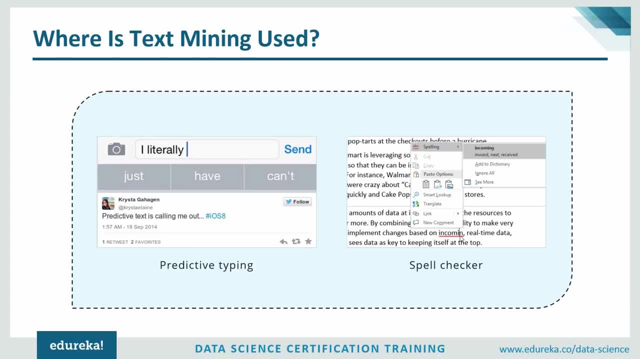 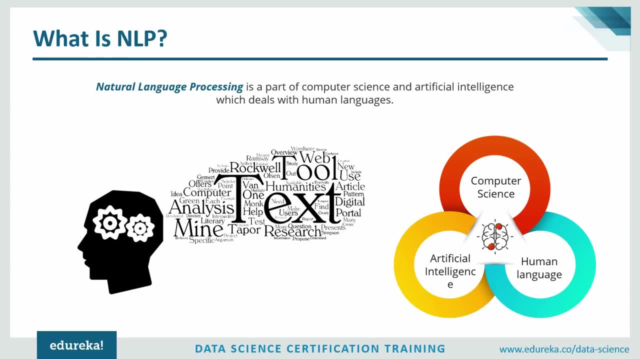 simple examples to show you how widely text mining is possible and how you can use text mining to use text mining. okay, now let's move ahead and discuss what nlp, or natural language processing, is. so, guys, a lot of people have asked me why is nlp and text mining considered as one and the same? 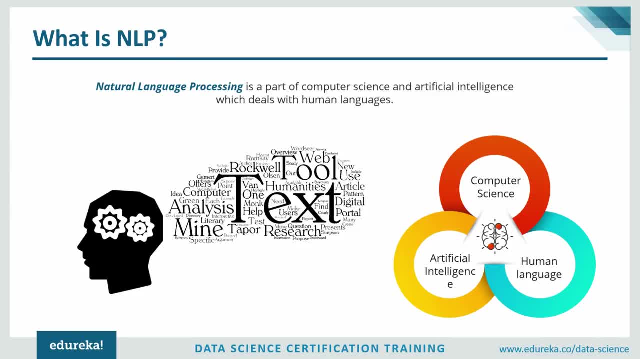 okay now nlp, which also stands for natural language processing, is a component of text mining, which basically helps a machine read the text. okay now guys. obviously machines don't actually know english or french. they interpret data in the form of zeros, only know binary form. so this is where nlp comes in. natural language processing is what computers 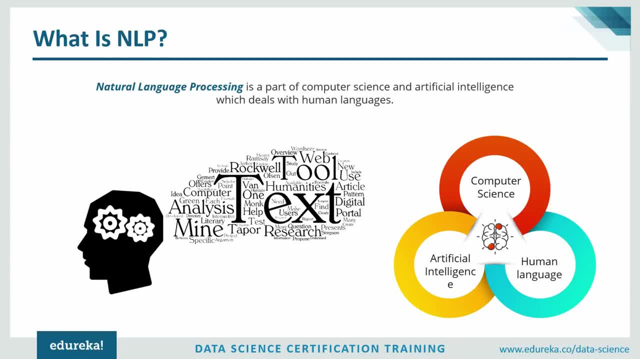 and smartphones use to understand our language- okay, both spoken and written. now, because we use language to interact with our devices, nlp became an integral part of our life. okay, nlp uses concepts of computer science and artificial intelligence to study the data and derive useful information from it. so, like i mentioned earlier, a lot of people are confused about the difference between: 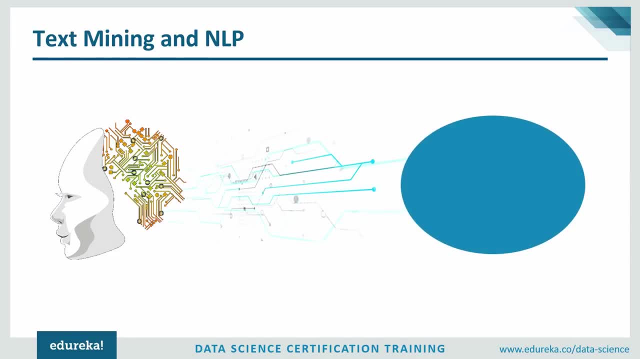 nlp and text mining. now, guys, text mining is a vast field that makes use of nlp to derive high quality information from the text. okay, so, basically, text mining is the process and nlp is a method to carry out text mining. i hope you have a clear distinction between the two. okay, now let's. 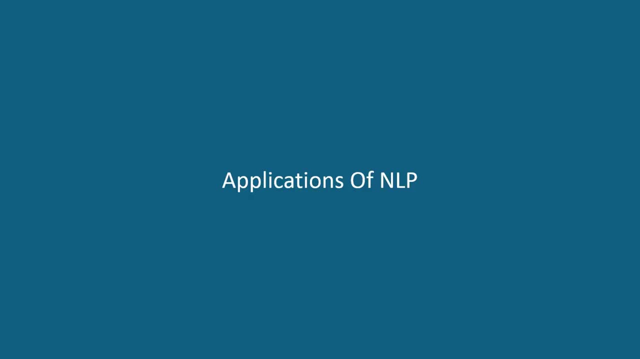 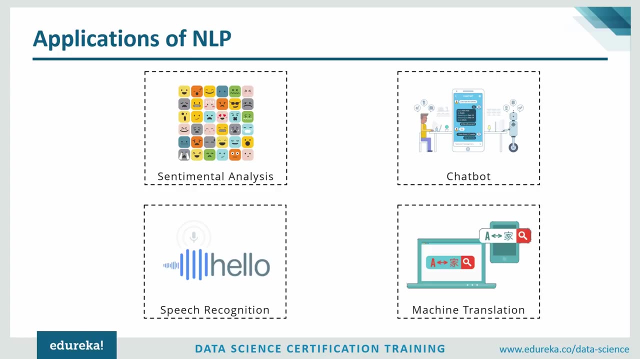 move ahead and take a look at the applications of nlp, or natural language processing. so first of all, we have sentimental analysis. so, guys, this is extremely useful in social media monitoring because it allows us to gain an overview of the wider public opinion behind certain topics. okay, 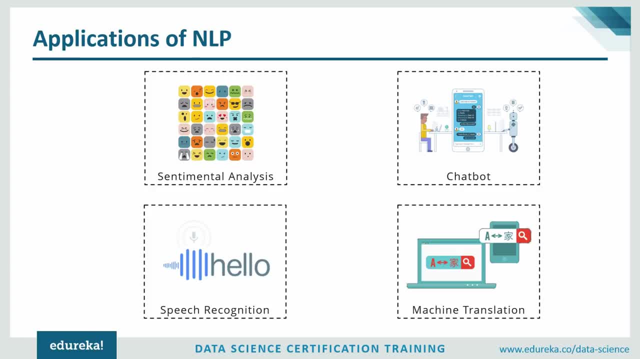 now, this application of nlp helps in growing business organizations. okay, they give them insights on what consumers like and what they don't like. all right. next we have the chatbots. now, guys, chatbots are the solution for consumer frustration regarding customer care call assistance. all right, so companies like pizza hut, uber have actually 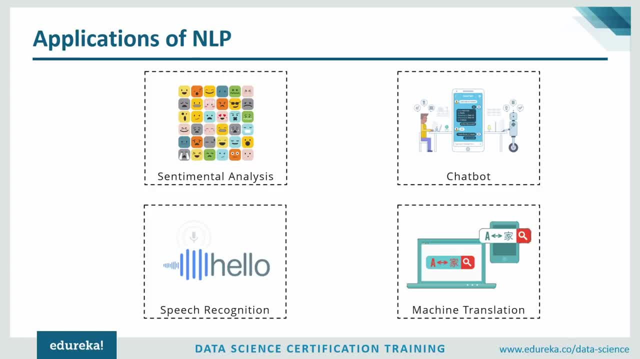 started using chatbots to provide good customer services. we also have something known as speech recognition. now, nlp has been widely used in speech recognition. we're all aware of alexa, siri, google assistant and cortana. now, these are all applications of nlp. machine translation is another. 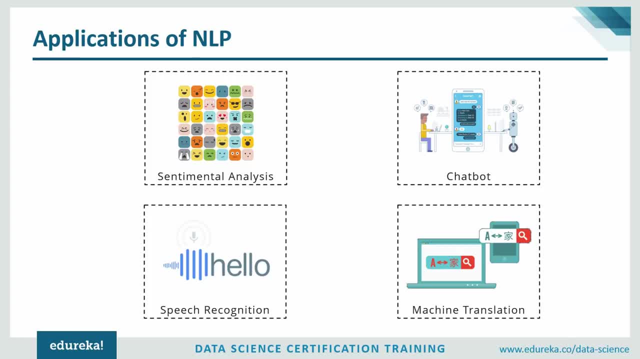 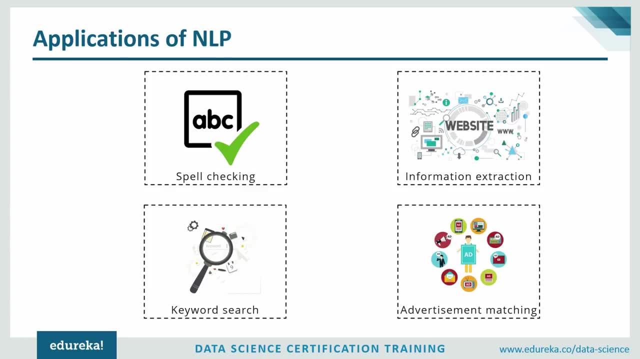 important application of nlp. an example of this is a google translator. all right, it uses nlp to process and translate one language to the other. other applications of nlp are the application of nlp, including spell checkers, keyword search, and there's also information extraction. now nlp can. 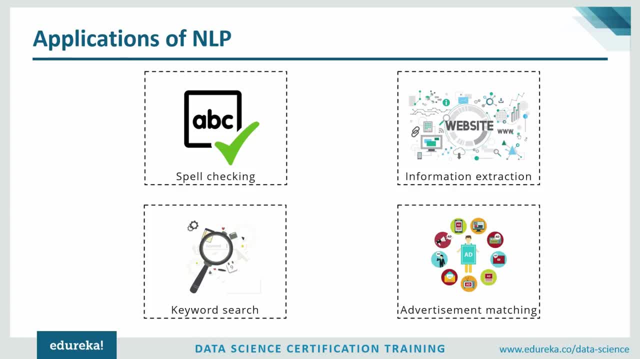 be used to get useful information from various websites or from word documents, files, and all of that. it is also used in the advertisement matching industry. now this basically means a recommendation of ads based on your history. all right, now that you all have a basic understanding of text mining and nlp, let's take a look at some of the important terminologies of text mining. so 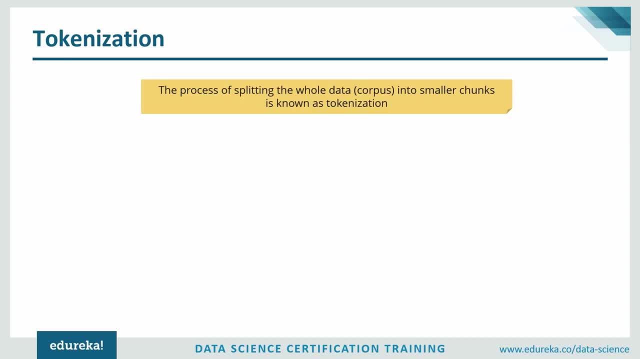 we're going to discuss about tokenization now, guys, tokenization is the most basic step in text mining. okay, it basically means breaking down data into smaller chunks or tokens so that they can be analyzed easily. all right, now let's take a look at an example. let's say i have this: 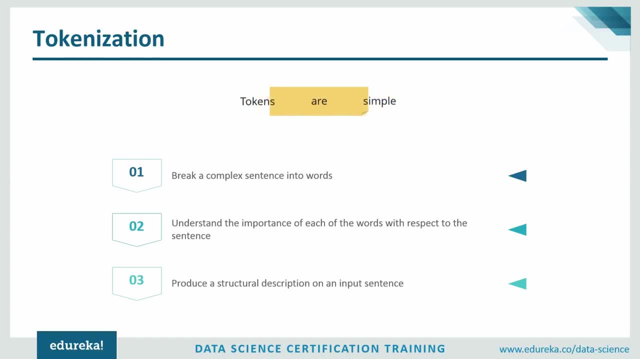 sentence, which is tokens, are simple. now, tokenization is basically breaking a complex sentence into words. then you understand the importance of each of these words with respect to the sentence, and then you'll use this information to produce a structural description on the input sentence. all right, so each of these are basically called tokens and tokenization is. 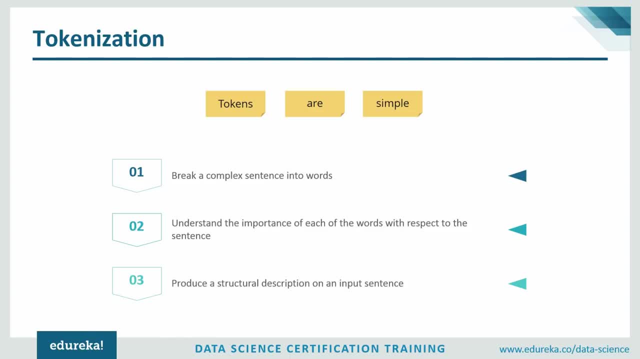 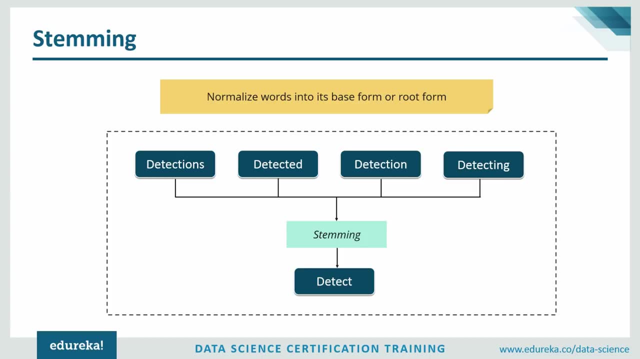 a process of breaking a complex sentence or a complex data into smaller chunks. all right, so the next terminology is stemming. so let's look at this example. okay, we have words like detections, detected, detection and detecting. now we all know that the root word for all of these words 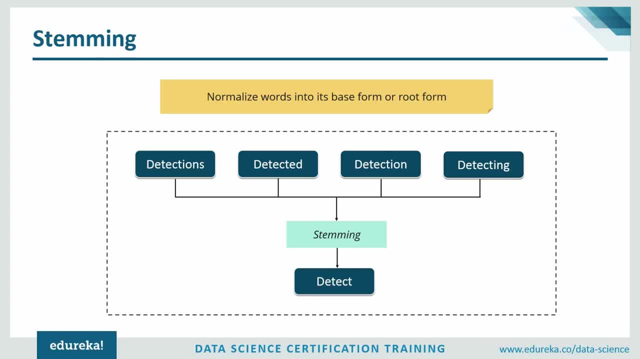 detect. so this is what stemming is about. stemming algorithms basically work by cutting off the end or the beginning of the word, taking into account a list of common prefixes and suffixes that can be found in an inflicted word. okay, now this process can be successful in some occasions. 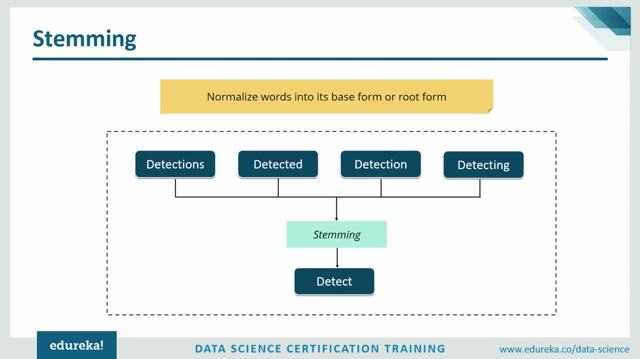 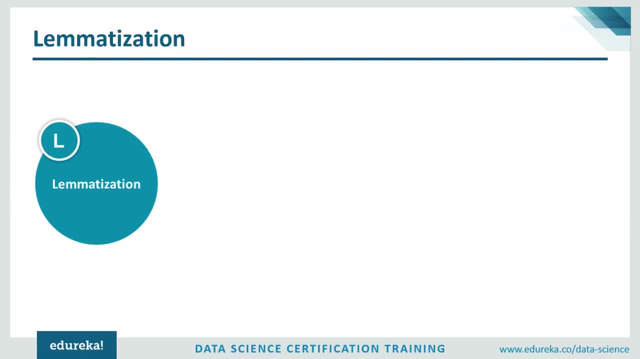 but it's not always correct, and this is why we affirm that this approach presents some limitations. all right, the next terminology is lemmatization. now, lemmatization is a better alternative to stemming. all right, now. what lemmatization does is it takes into. 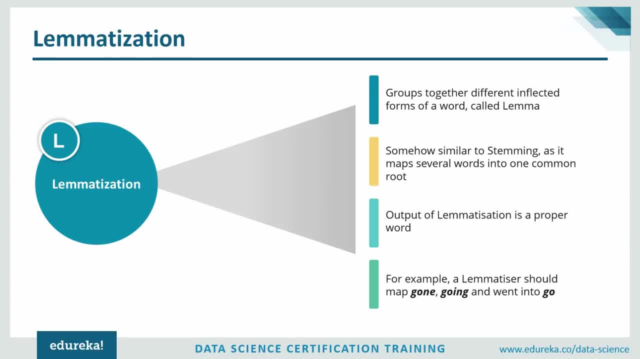 consideration the morphological analysis of the word. it is necessary to have detailed dictionaries which the algorithm can look through to link the form back to its lemma. okay, now let me just give you a small example. over here was like gone, going and went can all be written as go, correct, since 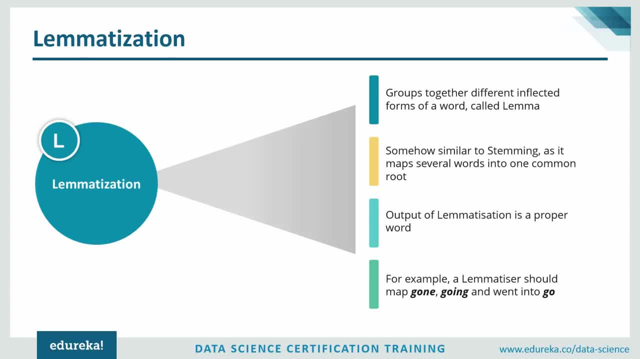 all of them actually mean the same thing. now, this is what lemmatization does. it doesn't actually cut prefix and the suffix of a word. instead, it goes through the meaning of the word. it takes into account the morphology of the word. okay, so it understands the word. 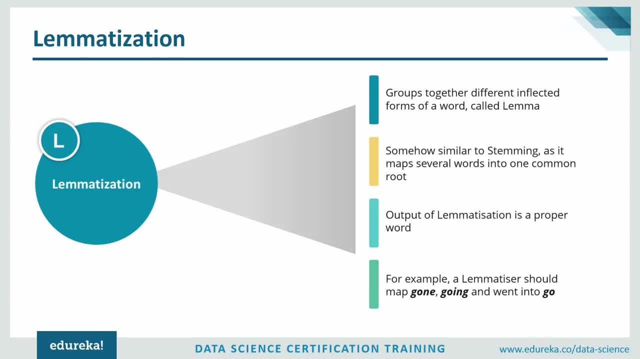 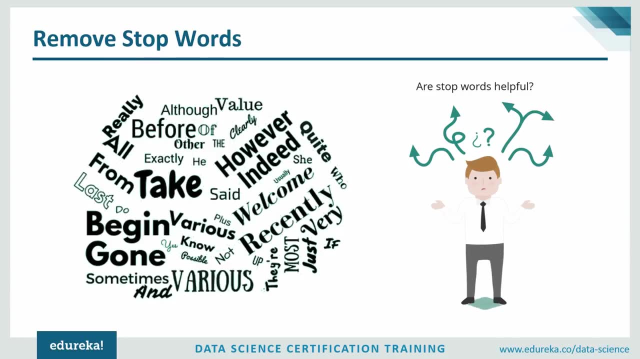 and only then it performs the lemmatization process. okay, this is a difference between stemming and lemmatization. all right, now let's look at our next topic. okay, so stop. words are basically a set of commonly used words in any language. so, guys, every language has this set of words that is used very. 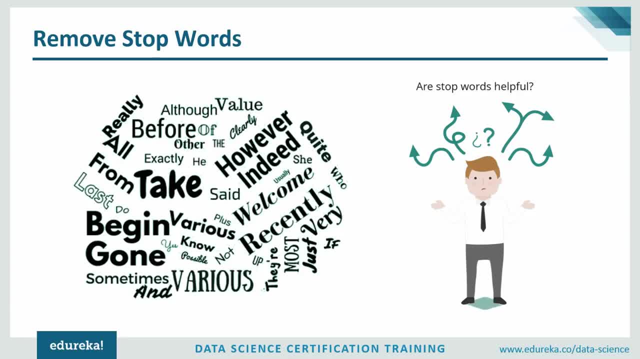 often. okay. so words like the- although value, before, after from all of these are very commonly used words. so what happens in text mining is, if we remove the words that are very commonly used in a given language, then we can finally focus on the important words instead. okay, so, for example, if I go to Google and search how 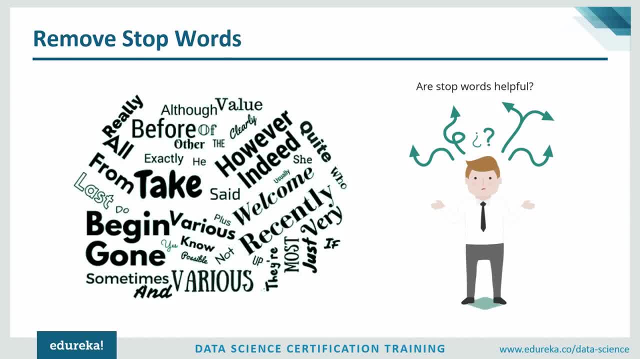 to learn text mining. now, if the search engine tries to find webpages that contain how to and learn, obviously the search engine will return a lot of pages, okay, that contain terms like how to and learn, instead of actually looking for pages which have text mining in it, okay. so that's why, if we disregard these three words, which is: 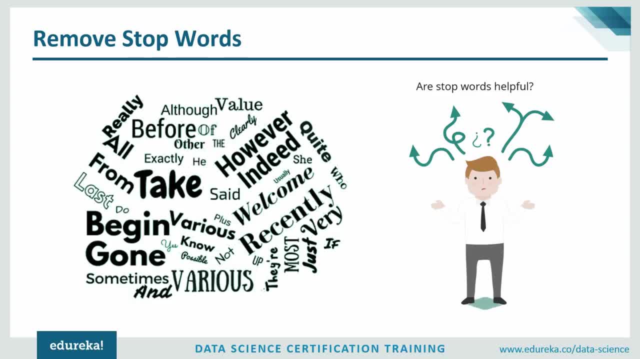 how to and learn, and we can actually let the search engine focus on retrieving pages that contain the keyword. okay, the keyword is text mining, all right. so, guys, that was all about stop words. it's quite necessary to remove stop words because you can finally focus on the. 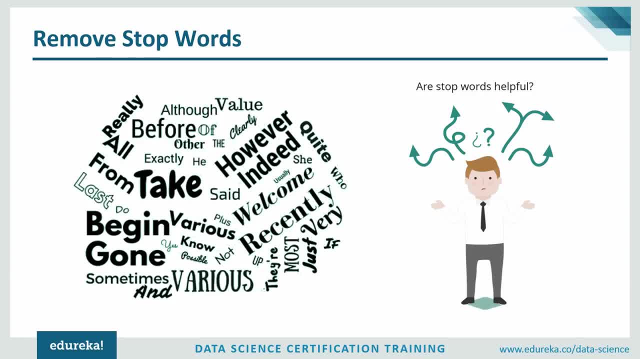 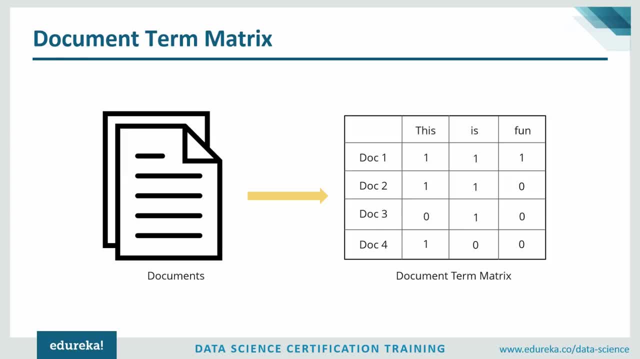 important ones, stuff. all right, now let's move ahead and look at our next terminology, which is document term matrix. so, guys, a dtm or a document term matrix basically has a rows filled with documents and the columns represent the words. okay, so if a word occurs in a particular document, then the matrix entry. 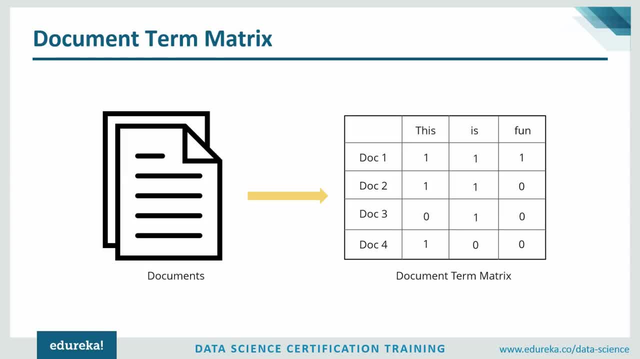 corresponding to that row and column is one. okay, otherwise it's zero. okay, so let's assume that we have a simple corpus now. corpus is basically a structured data set. okay, so if we have a data set containing four documents and we're trying to look for the frequencies of these three words, 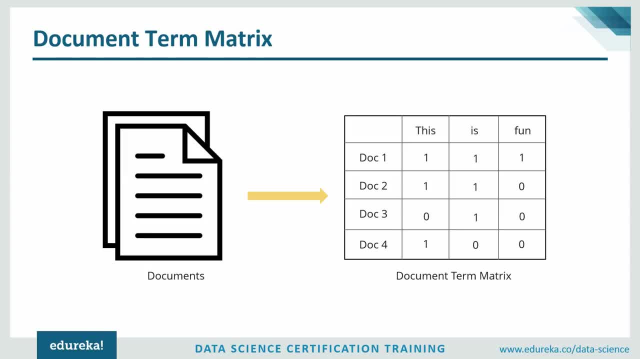 okay. so if document one had the word this, then a one would be put in the matrix. okay. similarly, if it has is, it's going to put one, and so on. okay, now, document two does not have fun, so that's why there is zero over here. all right, so, guys, this is what a document term matrix. 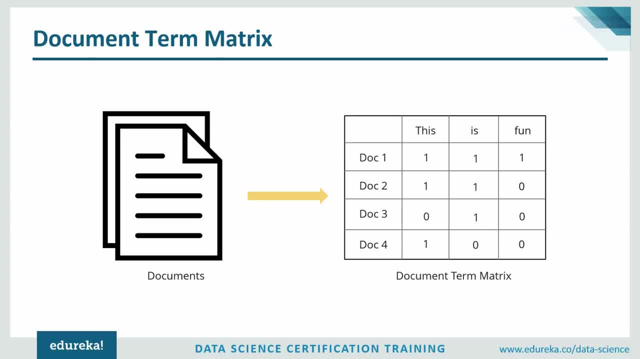 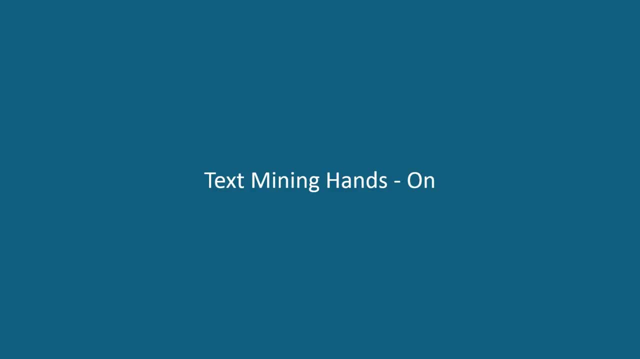 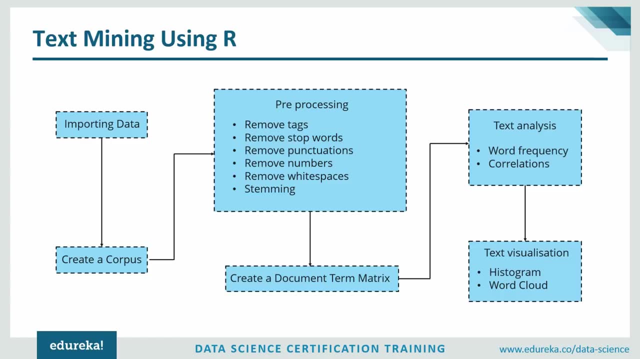 is. it's basically used for the frequency of words occurring in a document. all right, now let's get to the fun part. okay, so before we execute our demo, let me run you through what exactly we're going to be doing. okay, so for this demo, i have a bunch of documents on random topics. what we're going to 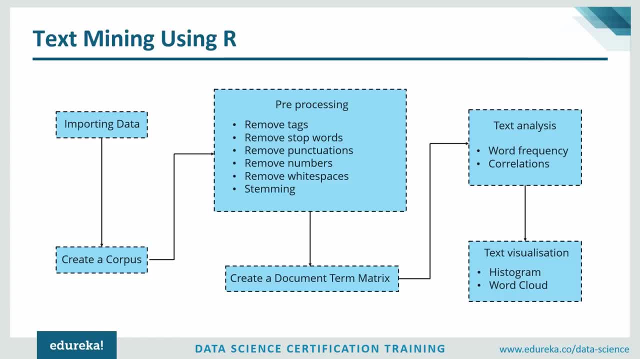 do is we're going to perform text mining on these documents, so we'll begin with importing the data correct and then we'll create a corpus out of it. so, like i mentioned earlier, corpus is basically a collection of documents. so we're going to do a collection of documents and we're going to 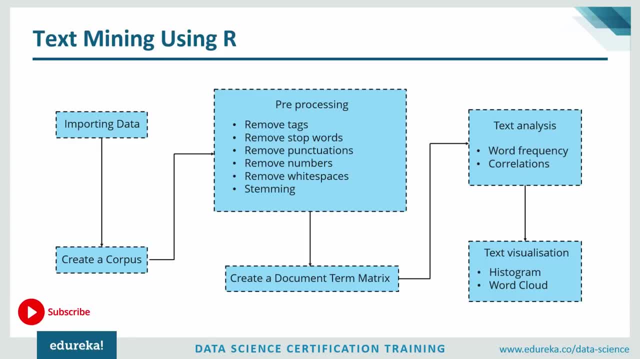 do a collection of texts. okay, a structured collection of text. after that we'll perform pre-processing. all right, this includes removal of tags, stop words, punctuations, numbers, white spaces and stemming. so after we've cleaned our data, we're going to create a document term matrix out of it. 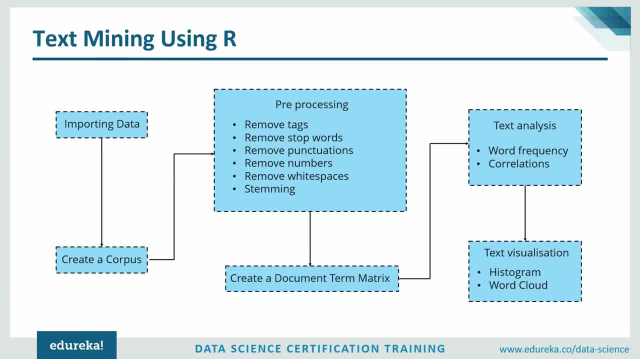 all right, then we're going to use the document term matrix in order to perform text analysis. here we'll check for word frequencies and word correlations, all right, and finally we'll end the demo by text visualization. we'll plot the data and then we're going to create a document term matrix. 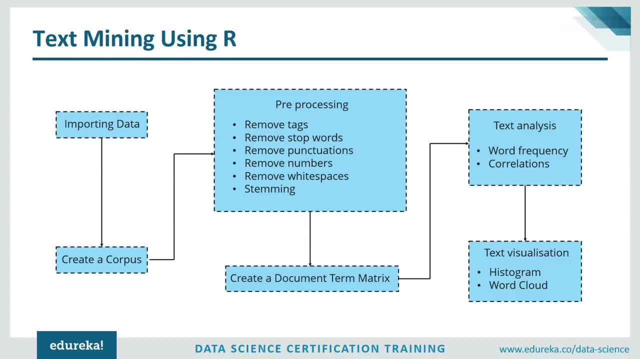 we'll plot a histogram to check the frequency of the text. we'll also create a word cloud. all right, since a lot of people are actually doing this, let's also try and create a word cloud. all right, now, without any further ado, let's move ahead to our demo. so, guys, in order to save some time, i've 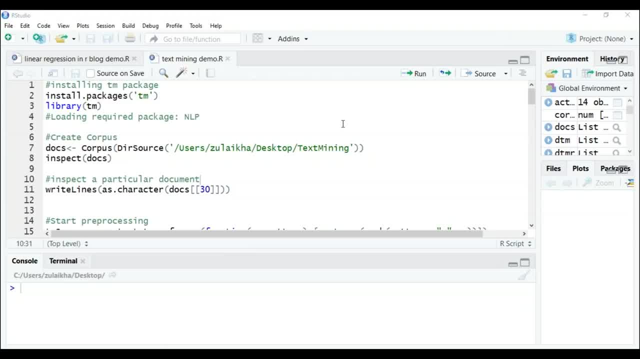 already typed the entire code and i'm assuming that all of you have a good understanding of r. all right, we're going to use the r language in order to perform text mining over here, so i'm not going to go too much in depth with explaining the code, but of course we're going to. 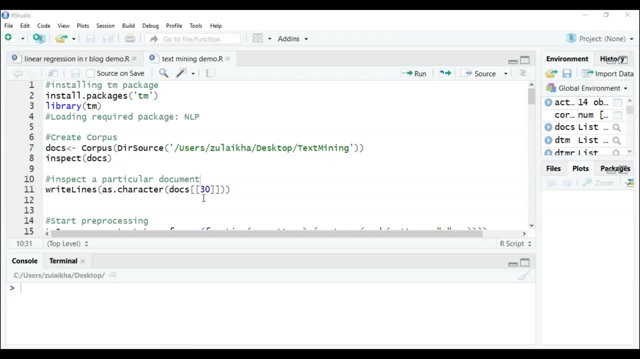 use the r language and of course i'll tell you what each line is doing. but i hope you all have a brief understanding of r, okay? if you don't have, then i'll leave a link in the description. you all can go through that video and then come back to this. all right, we're going to begin the demo by. 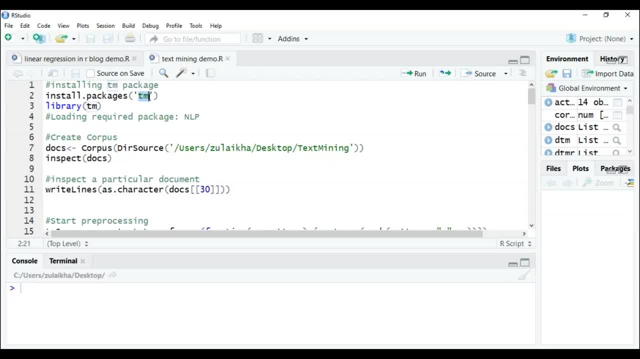 installing a package known as tm. okay, tm basically stands for text mining, and this package contains all the processes and all the packages that are required to perform text mining. okay, it's going to load our nlp package. so, guys, this is the advantage of using r and we're going to load our nlp package. 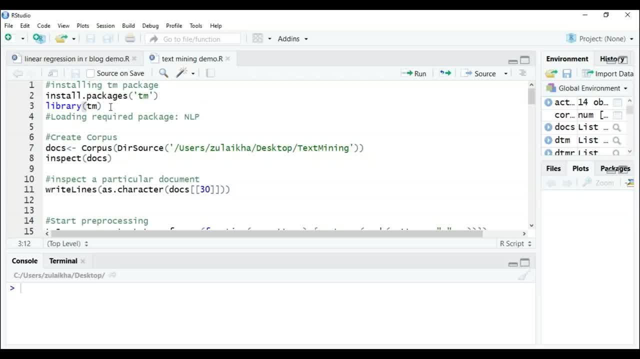 okay, r already has a lot of packages and libraries which perform all the functions for us. okay, so all we have to do is we have to install the package and then load the package. all right, so let's run these two commands. all right now. the next step for us to do is we need to create a collection. 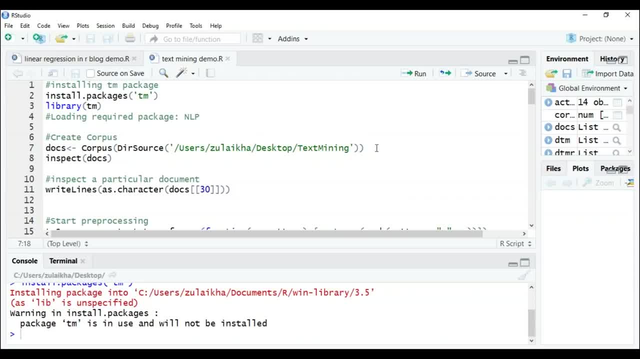 of documents. okay, now a collection of document is basically referred to as corpus in r. okay, i've created a folder known as text mining, within which i've stored all the data. okay, i've stored all my documents that we're going to be using in this demo, and i'm just giving a path. 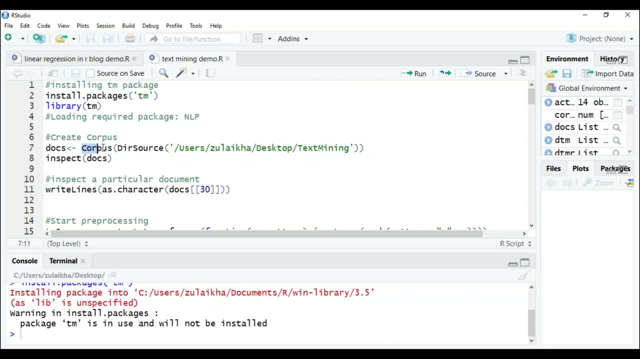 to that folder. okay, after that, you can see that i'm calling the corpus function. now this function is provided by the text mining package. all right, so i'm just calling the corpus function so that it can create a corpus out of all the documents in this folder. okay, and finally, i'm storing all of 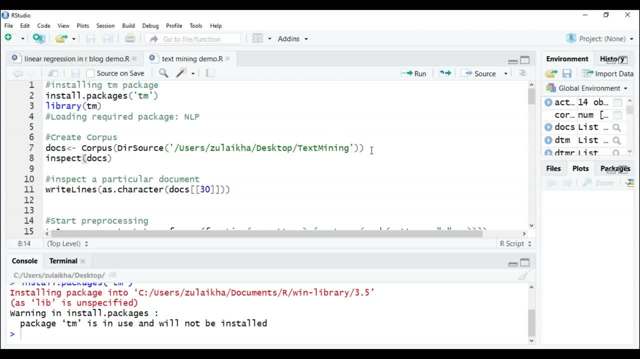 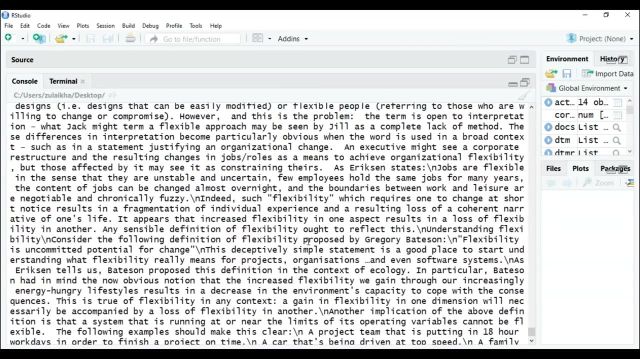 this in a variable known as docs. okay, so let's just run this line now. if you want to inspect the document, then run it. all right, so our document has loaded. okay, this is what the document looks like and i'm not going to bore you with this. so there are a lot of unnecessary things in this document. 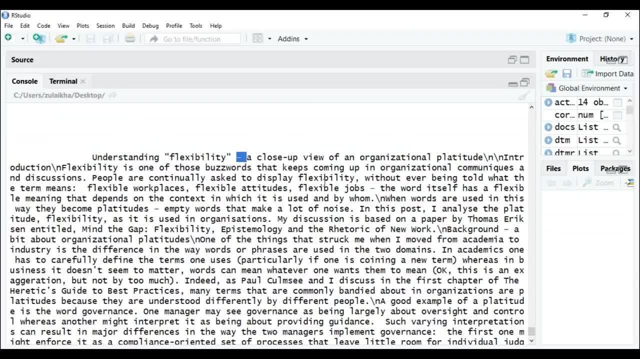 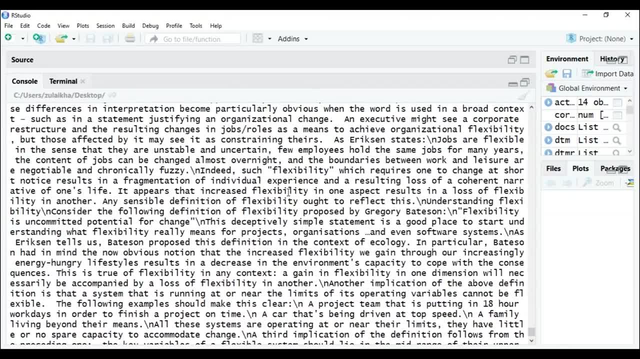 okay, we have a lot of quotation marks, we have a lot of hyphens, we have white space, we have backslashes. okay, we don't need all of this, and you know we'll be clearing all of this as we proceed in the demo. for now, let's move on to our next step. okay, so if you want to inspect, 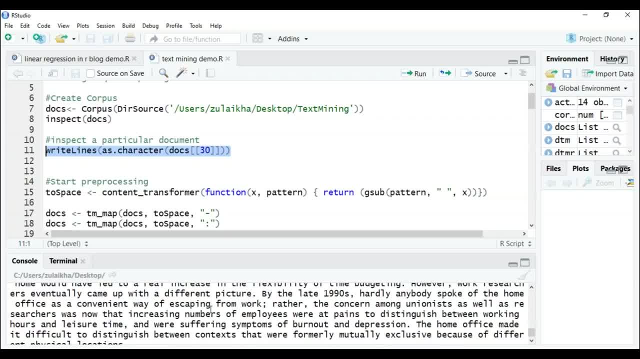 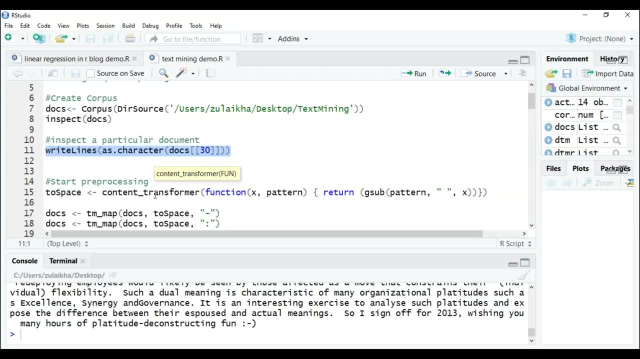 some particular document, then you can run this. okay, this will just give you one document out of all the documents that i have in my folder. all right, now let's start pre-processing. okay, so first of all, let me tell you something about pre-processing, or data cleaning. now data cleaning. 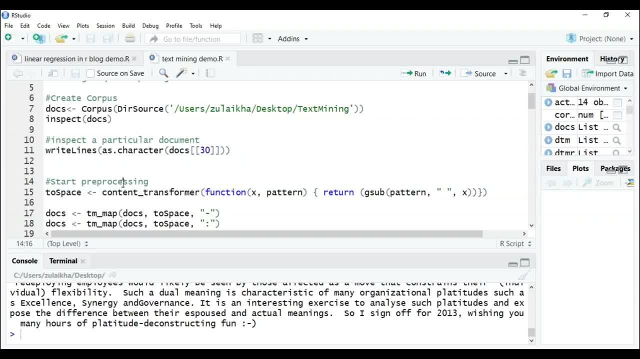 is a very important step in text analysis. okay, so, guys, if your data is not cleaned and if you you haven't actually removed the stop words, you haven't removed punctuations, you haven't removed the unnecessary part, then it's gonna be very hard to analyze such data. 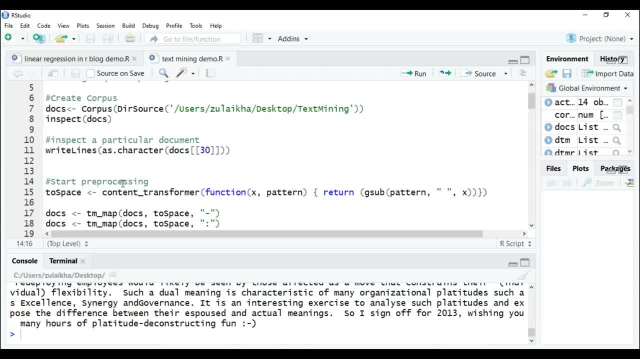 That's why data pre-processing is such an important step. Okay, this might be the most tedious step and the most time-consuming step, but this is essential in order to perform proper text mining, or proper text analysis. all right, So before we perform stemming and all of that, 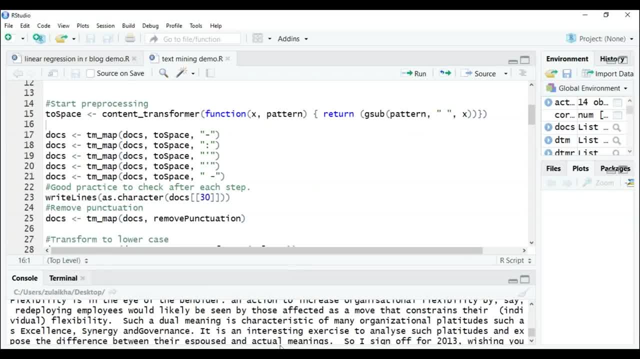 there are a few things that we need to take care of. So, guys, if you go through these documents properly, you'll notice that there are a few problems in the writing. For example, in the document they've used colons and hyphens. 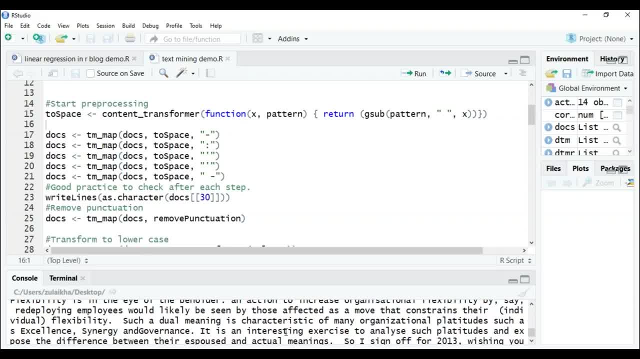 without adding any spaces between the words. okay, So if you use the remove punctuation transform without fixing this, this will cause the two words on either side of the hyphen or on either side of the colons to be combined into one word. okay. 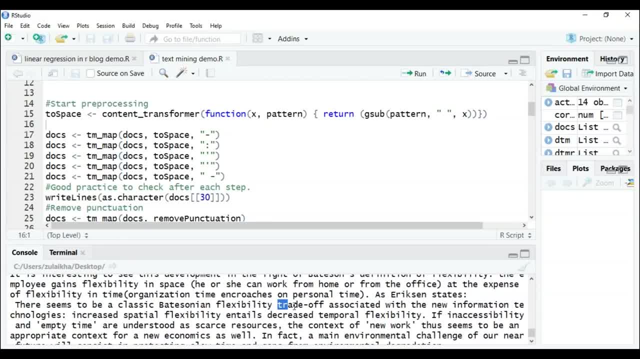 Let me show you a small example of this. all right, So, for example, we have this word over here: trade-off. So what I'm trying to say is this hyphen over here is used without adding spaces here. So if you use a remove punctuation function, 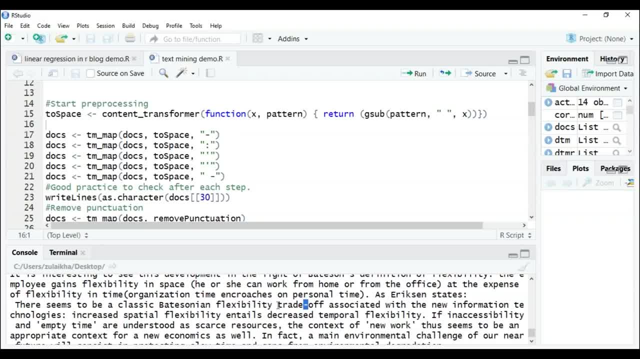 it's just going to remove this hyphen and it's going to make trade-off a single word, Okay. this is not going to make sense for a lot of words over here, So we need to fix this issue before we start using the remove punctuation function. 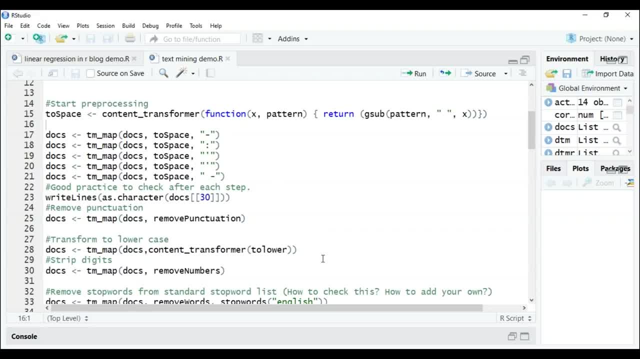 All right. To fix this kind of problem, all you have to do is you have to create a custom transformation function TM or the text mining pack which allows you to do this, by using a function known as content transformer. Okay, so this function will let us. 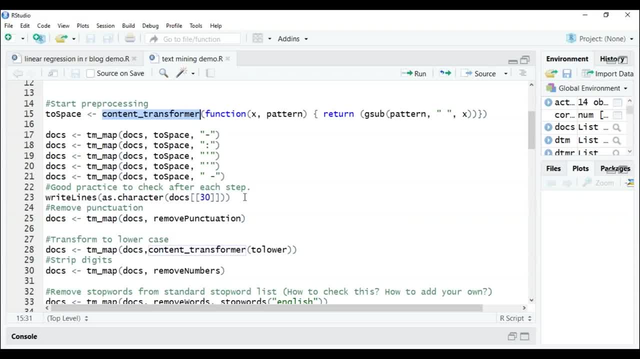 create our own custom functions and use them to clear off problems like these. okay, Now this function basically takes another function as an input. You can see this function over here, all right, So it takes a function as input and this function should specify. 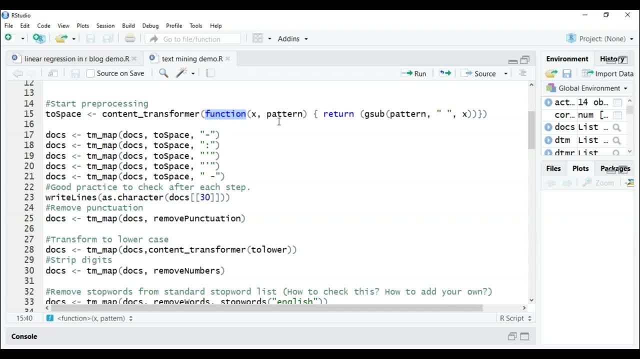 what transformation needs to be done. Okay, so, in this case, the input function would be one that replaces all the instance of a character by spaces. okay, So, here is a space that I've mentioned. okay, So, lucky for us, there is a function known as gsub. 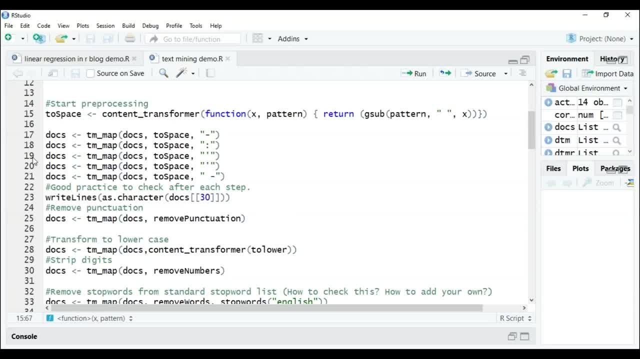 Okay, this function does exactly what I just mentioned. Okay, Now, this is basically the code to create the two-space content transformer. all right, So let's run this line of code. all right, Now you can use the two-space function. 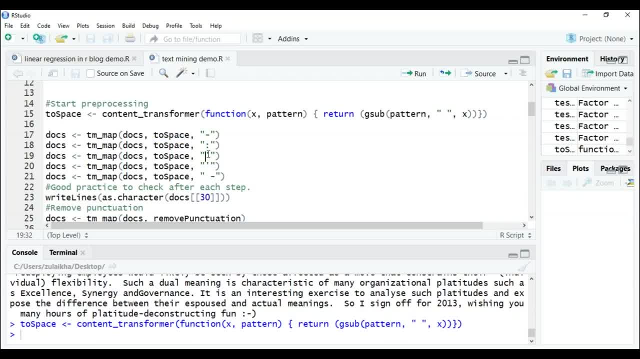 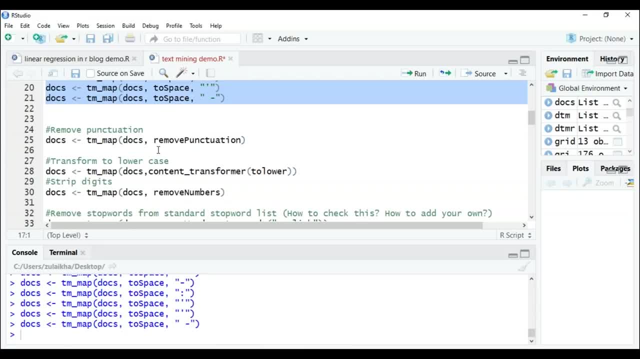 to remove all of hyphens, you can remove colons, you can remove single punctuations and all of that. okay, So let's run this entire thing. okay, So, now that we've done that, now we can finally use the remove punctuation function. 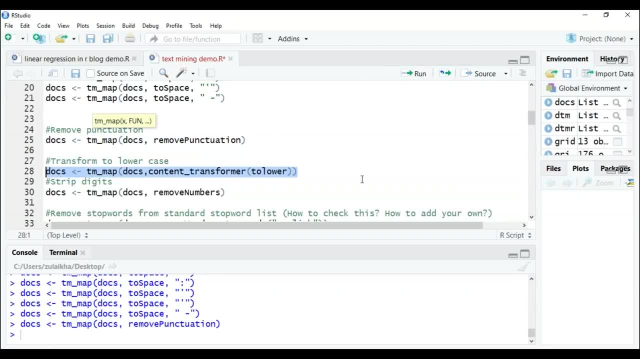 All right, so let's run this all right. After this, we're gonna go ahead and transform the entire corpus to lowercase. Now, why we're doing this is because R is case sensitive. Okay, so basically, if you have a word called text, 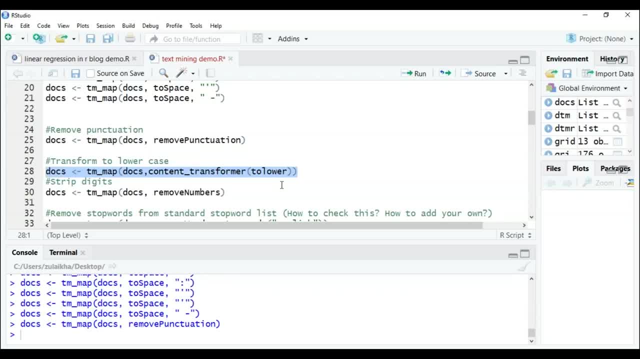 with a capital T and you have another word called text with cursive T. it's not going to consider it the same word. okay, It's going to think that the capital T text and the small t text are two different words, okay. 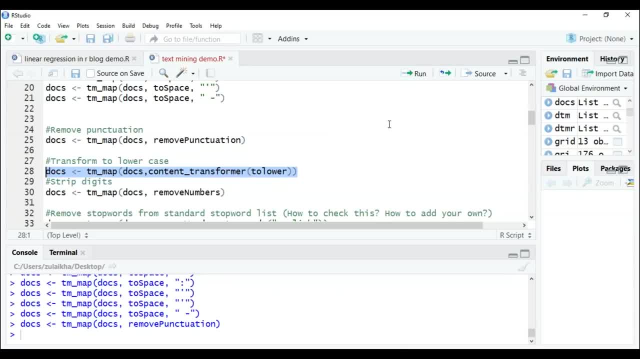 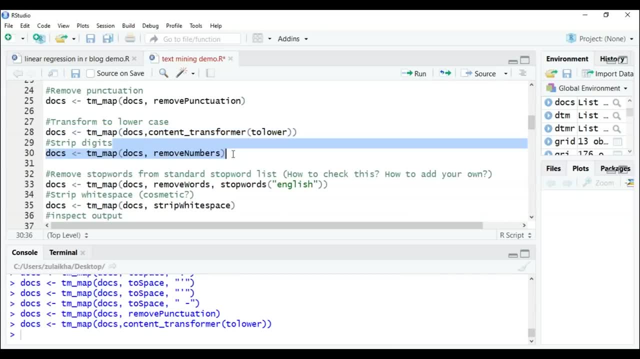 So, in order to get rid of problems like these, we're going to transform the entire text to lowercase. Okay, so let's do that. Next, we're going to remove any sort of numbers or any sort of digits. okay, Now, removing numbers is not something. 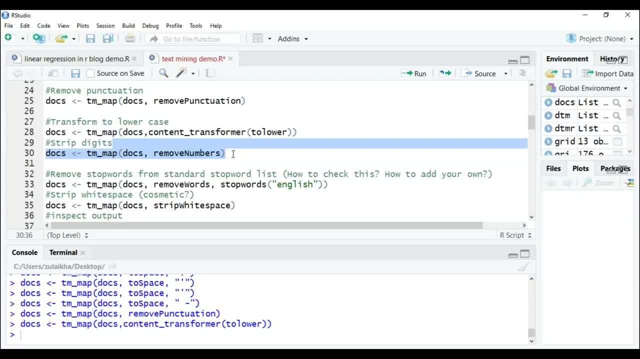 that you do every time. okay. So there are some particular cases wherein you need numbers in your text, But in our demo, we don't actually require any text because we're not going to perform anything related to it. Okay, that's why I'm removing any sort of numbers. 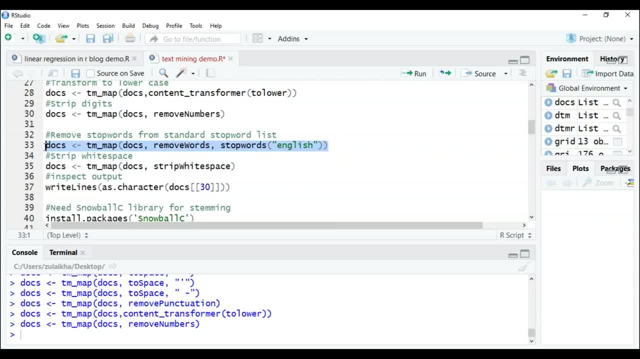 All right. Now the next step is to remove common words from the text. These include words such as and, the a, and conjunctions like and, or, but, and all of that, okay. You can also remove common verbs like is, yet. 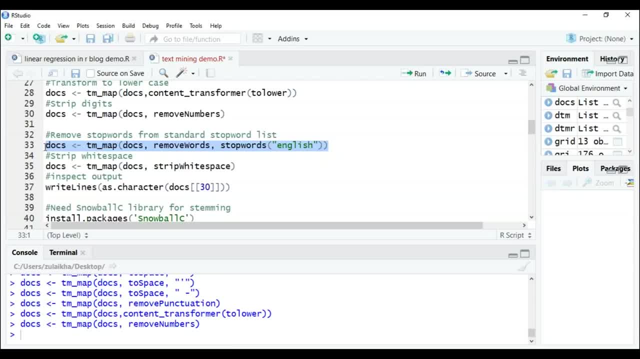 and all of that, Okay, all of this. yet, however, before, after, all of these words will get removed. okay, All of these words will get removed, okay, by using the stop word function. okay, So, guys, again the PM package or the text mining package. 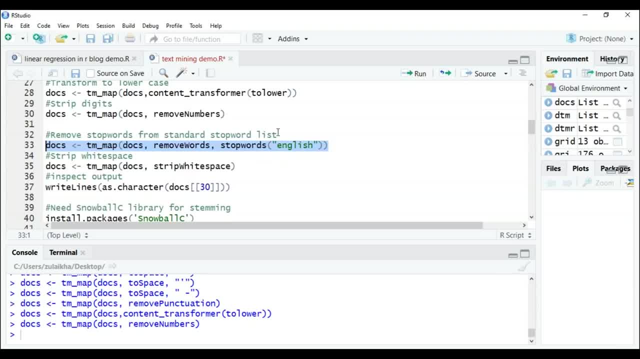 has a list of stop words. okay, So whenever you give a function stop words, it's going to remove all of the words in that list. Now let's run this line of code And finally we'll remove any sort of extra or extraneous white spaces. okay. 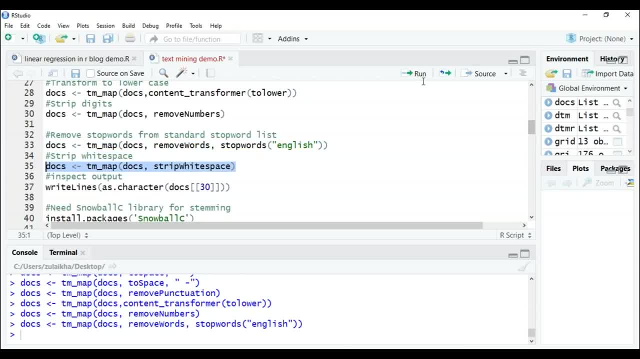 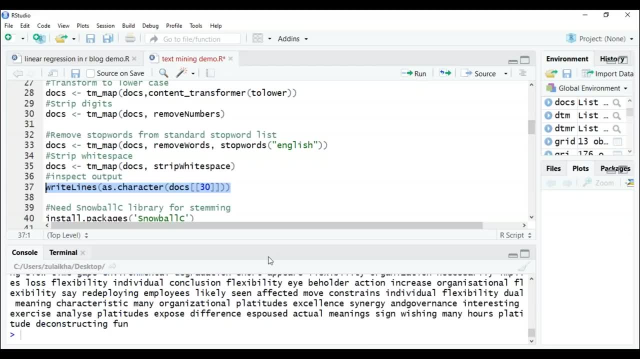 So we'll use a strip white space function to do that. So let's run this line And now let's inspect our document. okay, Now that we perform so much of text mining, let's see if our document looks okay. I don't see any hyphen. 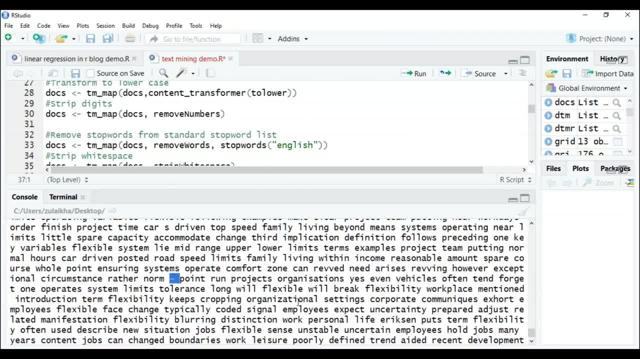 Okay, so far I do not see. Okay, I see one over here Now, guys, this is the problem or this is a limitation when it comes to using such functions. So, guys, text mining is an iterative process. Okay, you can't just do it once and leave it. 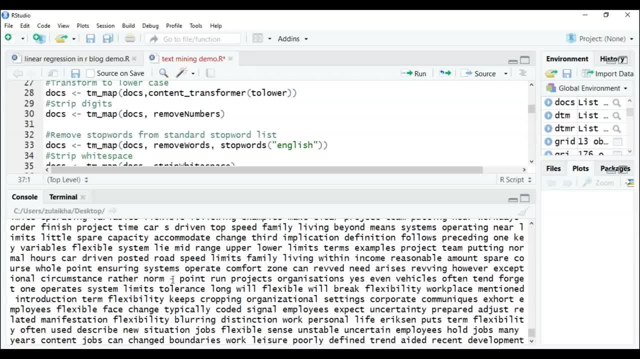 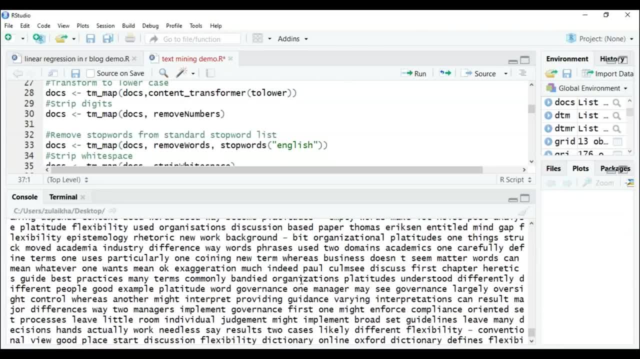 You have to keep doing all of this again and again in order to remove any unnecessary word or anything that was missed out in the previous time. alright, All right. from that, I think everything looks fine to me. okay and nothing. I don't see any capital word. 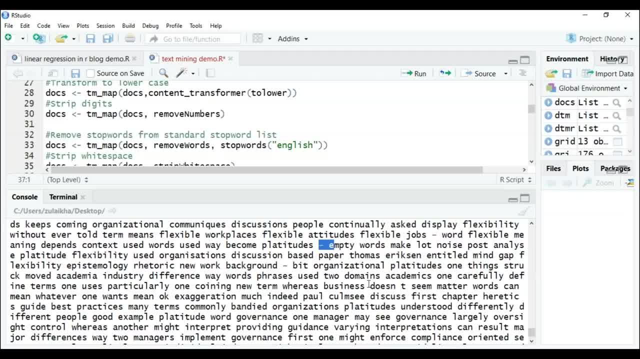 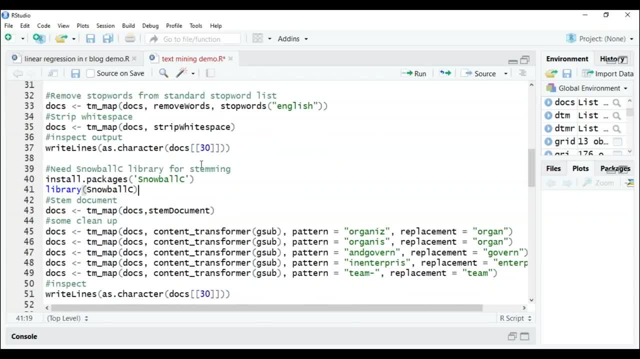 or anything like that. I do see a few hyphens, though. okay, it looks good. all right, now let's move on and perform our next step, which is stemming. okay now, before we actually perform stemming, I want to tell you that the library or the package that is needed to perform stemming, 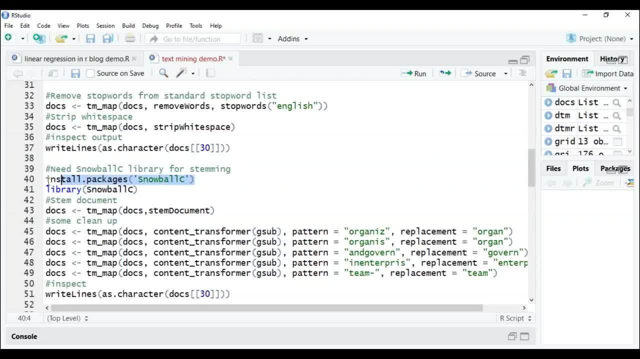 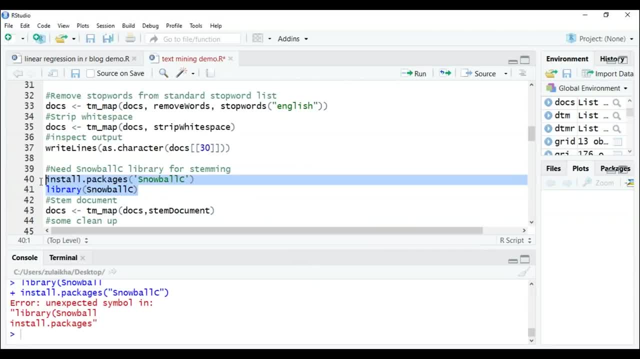 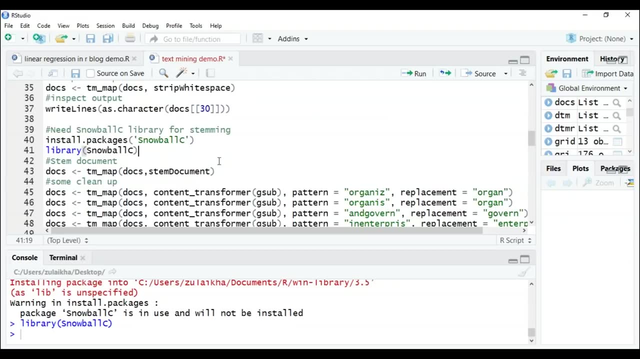 is known as snowball c. okay, so first you have to go ahead and install the package and then you have to load the package. all right, so let's perform that first. I did not select the entire thing, so I got a small error. okay, so now I've loaded the snowball c library into my R studio. now what I'm? 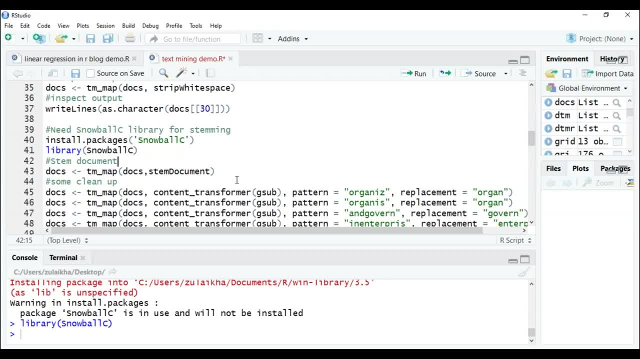 going to do is now I'm going to perform stemming. okay so, guys, like I mentioned earlier, there are a lot of words which have unnecessary prefix and suffixes. okay, so, words like detection, detecting, detected- all of this can be cut down to detect. okay, so this is exactly. 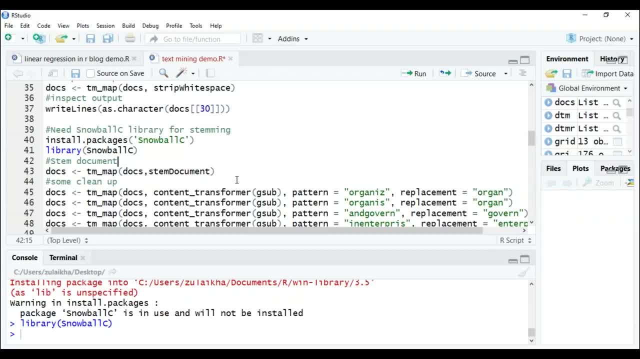 what I'm going to do. okay, so I'm going to go ahead and install the package, all right, so let's see what stemming does. but the thing with stemming is, I said it has a few limitations. all right, it might cut off prefix and suffix of a few words, which we do not want. okay, because 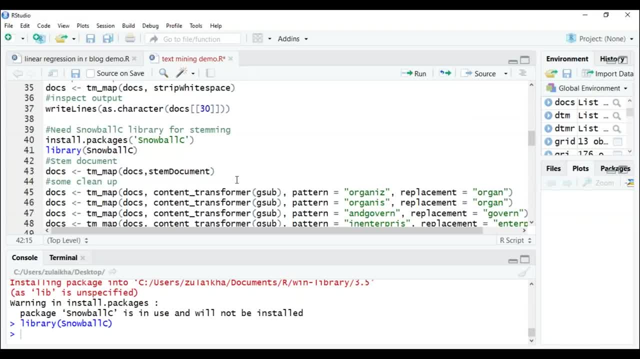 some words do not make sense without the prefix and the suffix. okay, so performing stemming is something that's optional. okay, it's left to you if you want to do it, but I'm going to go ahead and just show you how this is done. okay, now, before I perform stemming, I want you all to 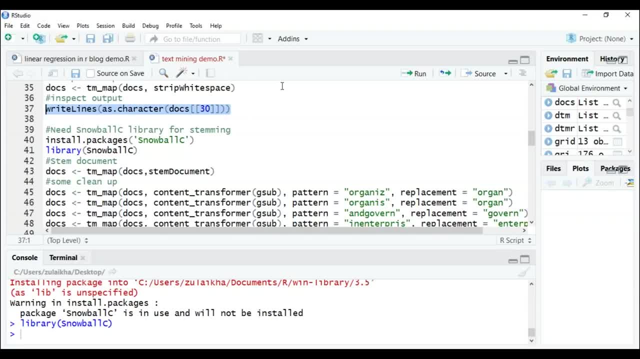 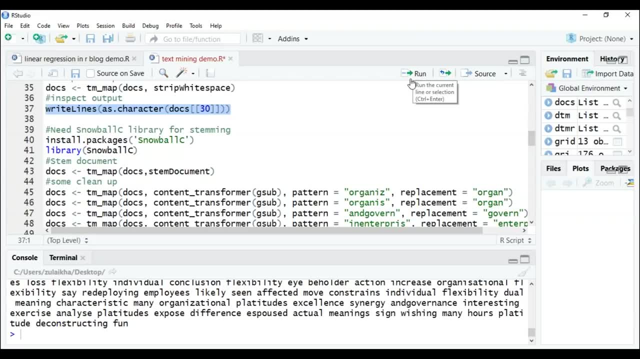 go through the last few sentences of our document, okay, so that you know what stemming really does. okay, and I can also show you the limitations of stemming through this. so let's go through the last few lines. okay, so this is what the last few lines look like without stemming. now let's perform some stemming on this. okay, now let's view our document. 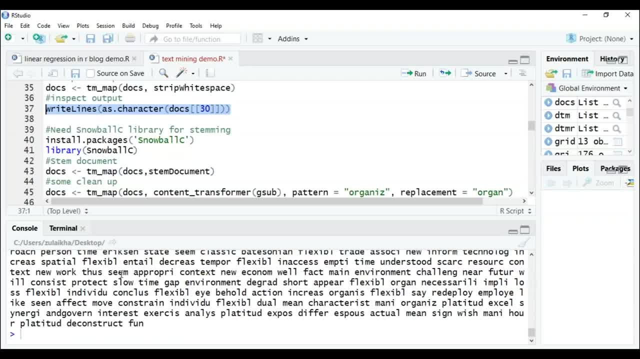 and let's compare, okay. so here you can see that a flexible has been cut down to flexible without an E, okay. exercise also is being cut down and Analyze has also been cut down- okay, There are a lot of things that we don't actually want, okay. 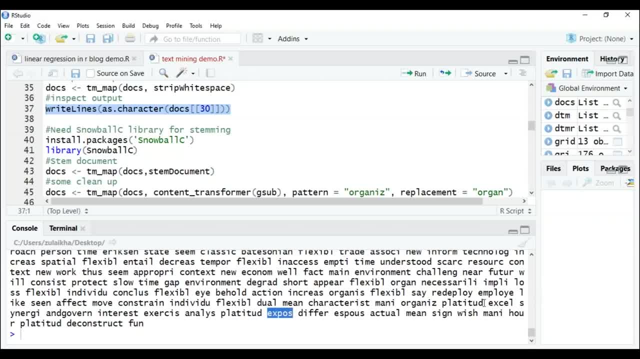 So I don't know what expose. I think this is supposed to be. expose. all right, This as well. this too: Organ, or I think organization, has been cut down to organ or something like that, I'm not sure. Okay, so, guys, this is the downside of stemming. 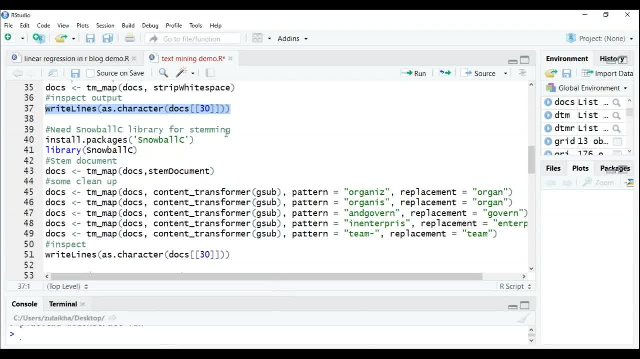 Now in our document. it's very evident Now: in a lot of cases, stemming is actually considered very important and crucial because they do not care about the English formatting of the text. okay. Instead, they want to perform text analysis for different reasons. okay. 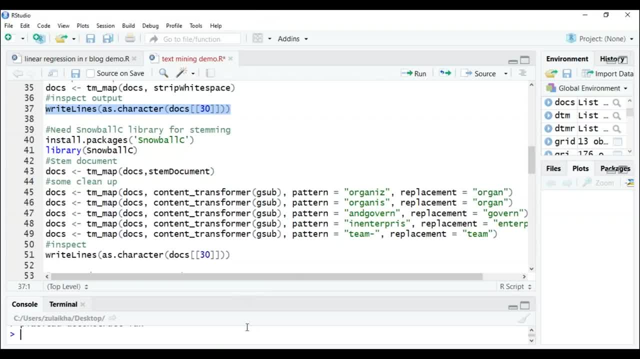 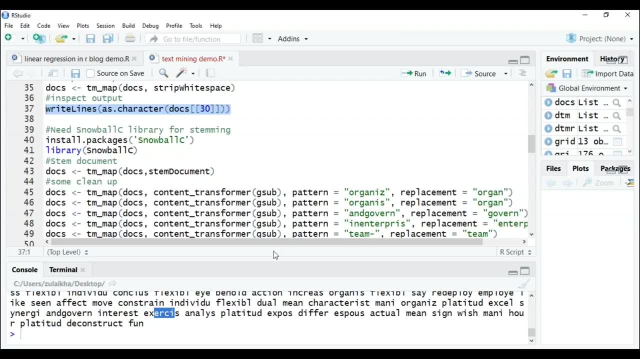 So their stemming is important. Now here, clearly, stemming is not a lot of help for us, because it's cutting down a lot of words that I don't want it to. okay, Now, I was just doing this in order to show you how stemming works. 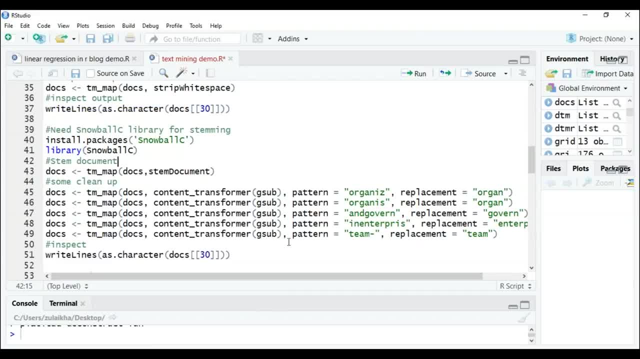 But now let's move on and do some cleanup, okay. So I've realized that in the document a few words have been cut down better, Very oddly, okay. So I'm going to replace those words. I've just added the replacement over here, okay. 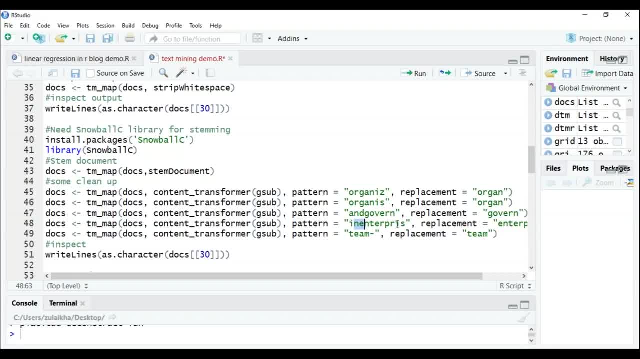 For example, and govern is cut down to govern In enterprise is enterprise Team with a hyphen is team. okay, So I'm just going to perform those cleanup over here. all right, That's done okay. So if you want to inspect the document, we can run the code. 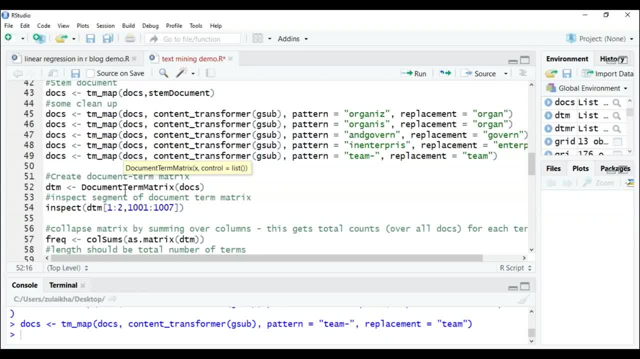 Now the next step to do is to create a document term matrix. okay, Initially, I told you all that it's basically a matrix which checks the frequency of words. all right, So it's going to have all the documents arranged in the row. 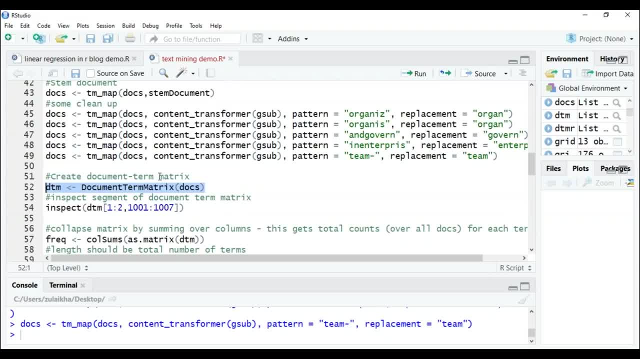 and all the words arranged in columns. So let's use the document term matrix function in order to create a DTM. okay, If you want to view the entire matrix, you can do that, But the thing is, this matrix is going to be very sparse, okay. 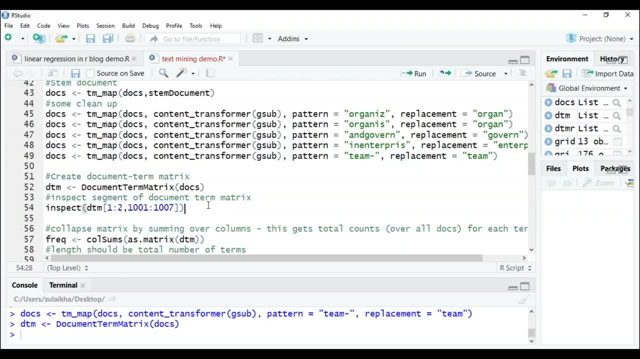 There are a lot of words which are not there in a few documents, So most of the matrix is going to look like zeros to you instead of you know having ones in it. Okay, so let's just inspect a part of it. 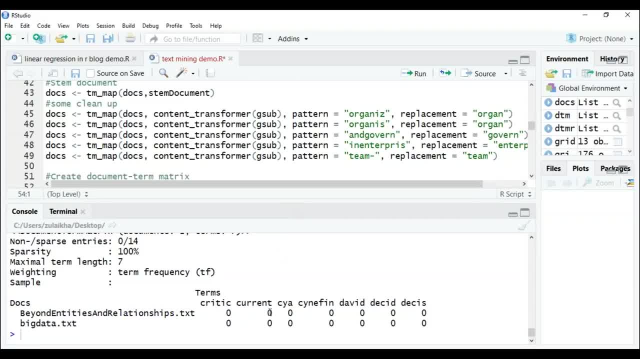 in order to show you what it looks like. okay, So here again, you can see only zeros. okay, So the sparsity of the matrix is 100%. okay, There are a lot of documents in my file and clearly these two documents do not have these words. okay, 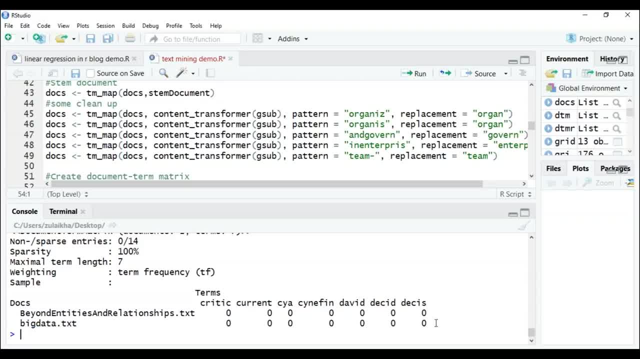 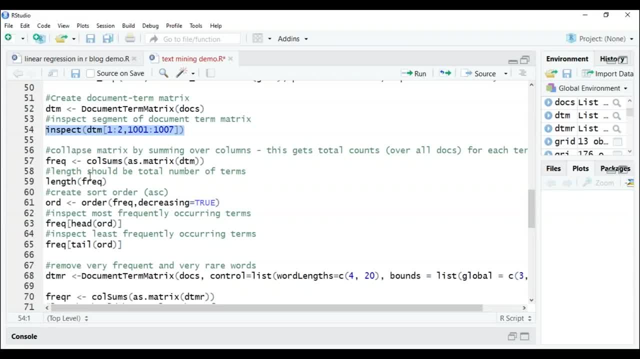 They do not have these words. That's why there is a zero corresponding to all of these rows and columns. all right, So now that we have created a document term matrix, we can finally perform analysis. Notice that after you construct a DTM. 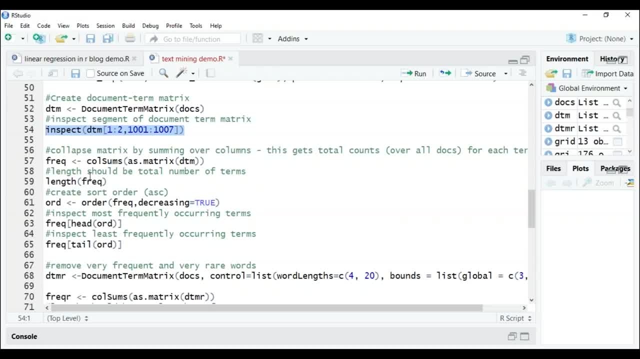 we have actually converted our entire corpus into a mathematical object. okay, Now this object, or this mathematical matrix, can now be analyzed using quantitative techniques. okay, So, guys, this is where the text analysis part starts. okay, So, for example, if you want to get the frequency, 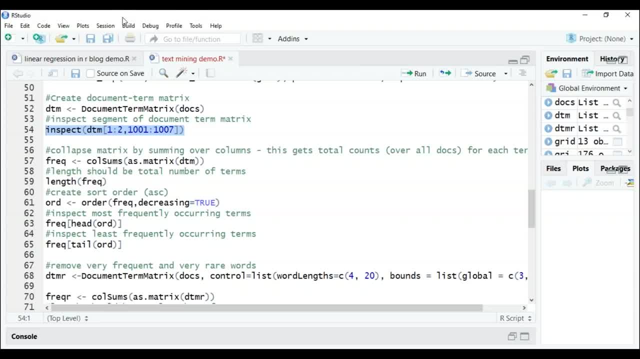 of occurrence of each word in the corpus. what you're going to do is you're going to simply sum over all the rows to give you the column sums. okay, That's exactly what I'm going to do, So let's go ahead and do that. 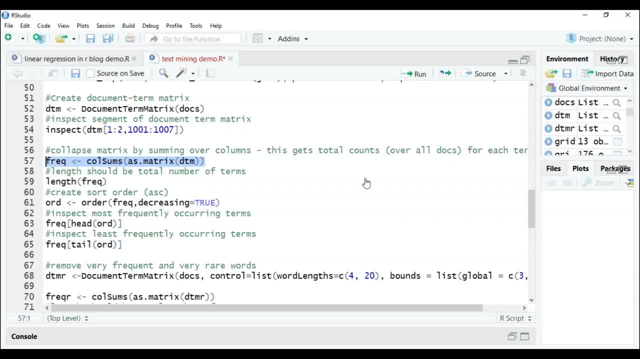 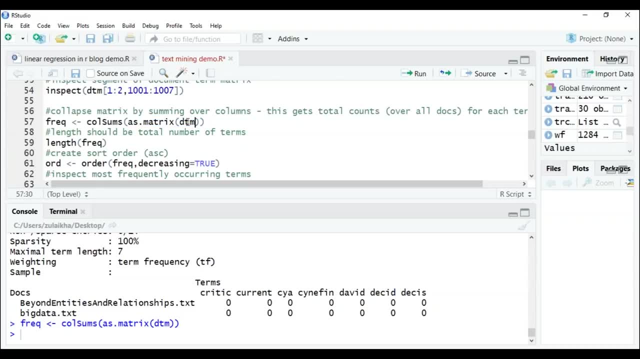 So let's go ahead and do that. So let's go ahead and do that. So if I run this line, it's going to give me the frequencies, all right. Now, if you notice this line properly, what I'm doing exactly over here is we're converting the DTM. 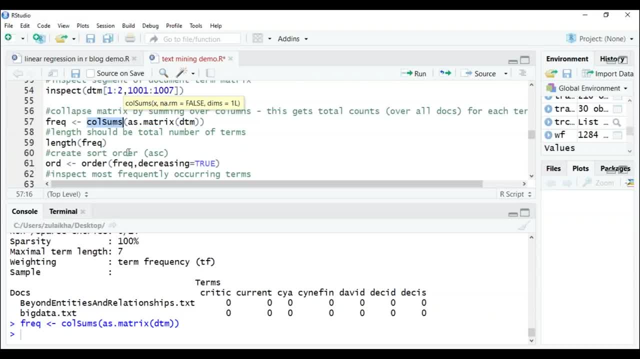 into a mathematical matrix, and then we've just summed over all the rows to give us the total of each column or each term. okay, Now, whatever the result is there, it's going to be stored in this frequency variable. okay, So you can go ahead and inspect the variable. 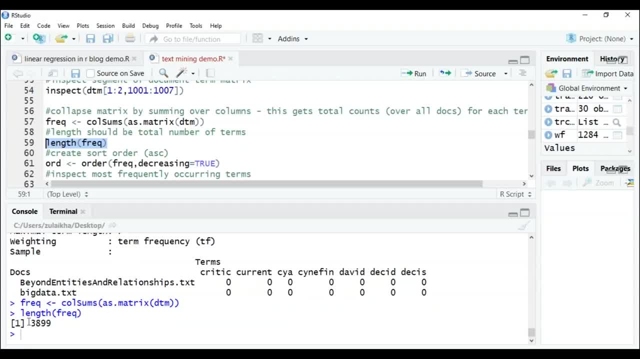 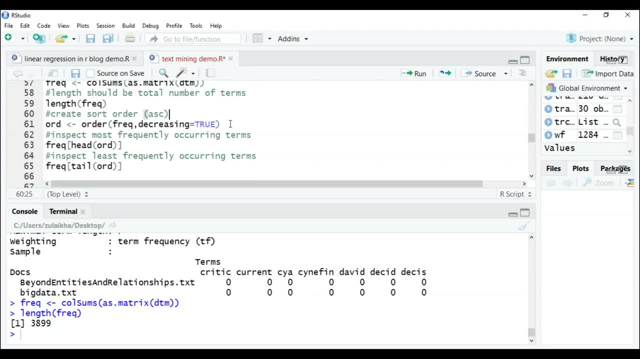 or you can just check the length using the length function. Okay, this shows us the length. That is 3,899,. all right. Next, what we're going to do is we're going to sort the frequencies in descending order. We're going to start with the most frequent word. 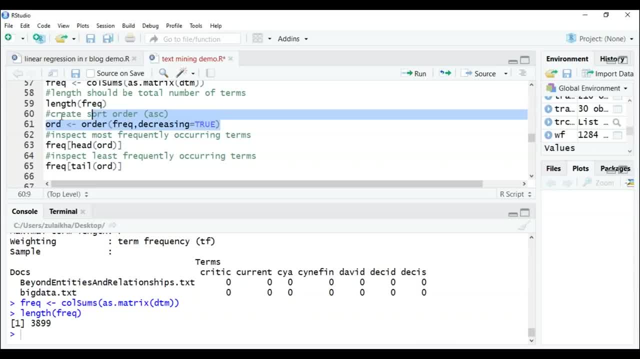 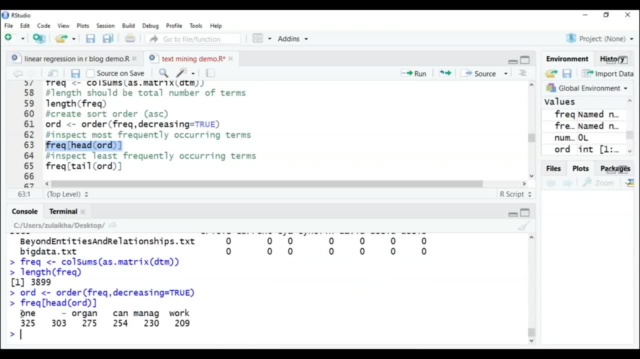 and we're going to end up with the least one. okay, So let's run this line of code. So if you want to inspect the frequencies of the first five elements, you can do that. So you can see over here: one occurs 325 times. 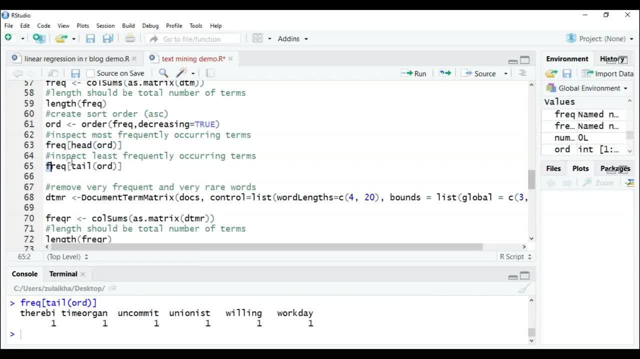 So you can either check the most frequent words or you can also check the least frequent words. This will just give us a list of least frequent words, okay, So if you run that. so uncommit occurs only once, unionist occurs once, billing occurs once. 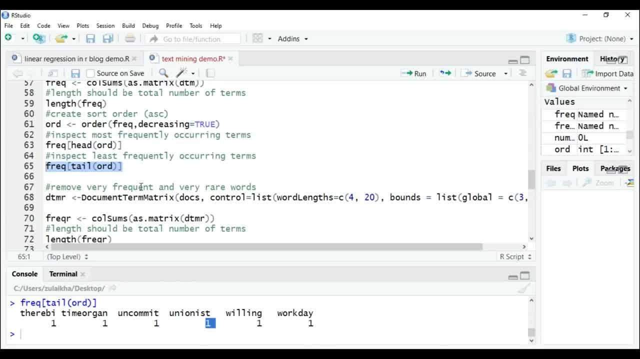 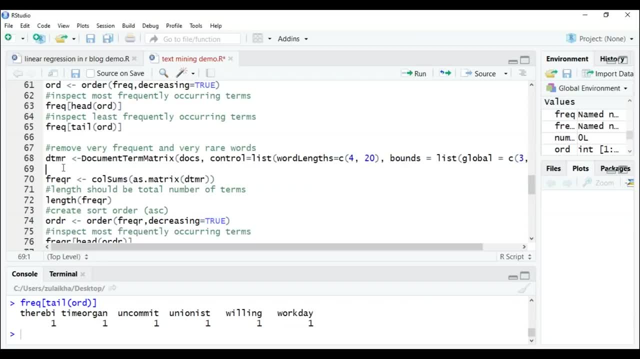 and workday occurs once. okay, So these are the least frequent words in our documents. So, guys, the thing to note over here is that the least frequent terms are very interesting, okay. Now, this is because the terms that occur very rarely, 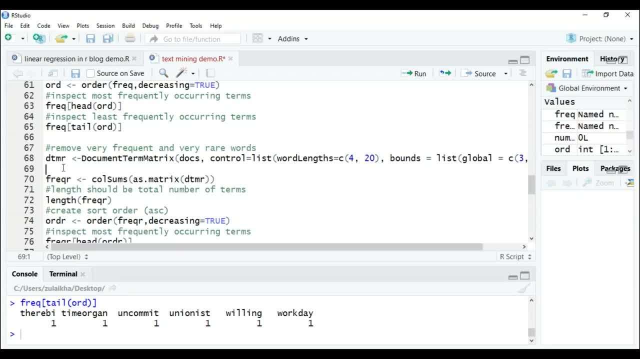 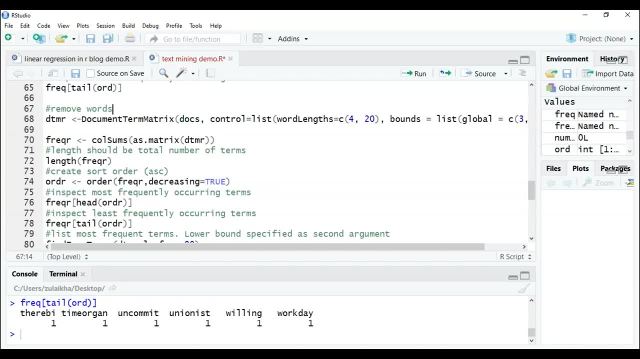 are likely to be more descriptive of a specific document. okay, Okay, So the least frequent words are given a lot of importance. okay, Now, guys, there are a lot of words like can, like one and how. all of these words give us no information. 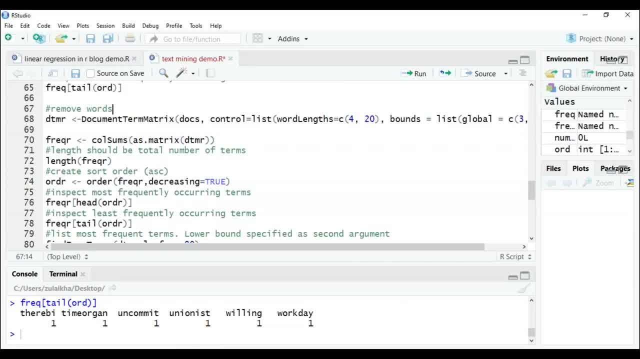 about the subject. okay, They give us no information about our document at all, So that's why we can eliminate such words. okay, And I know that we've performed the stop word analysis wherein we removed all the stop words, but I told you earlier. 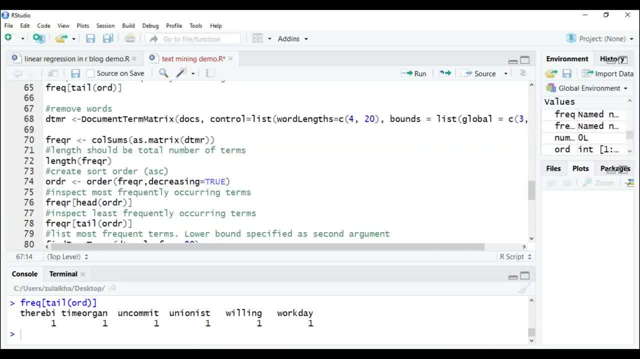 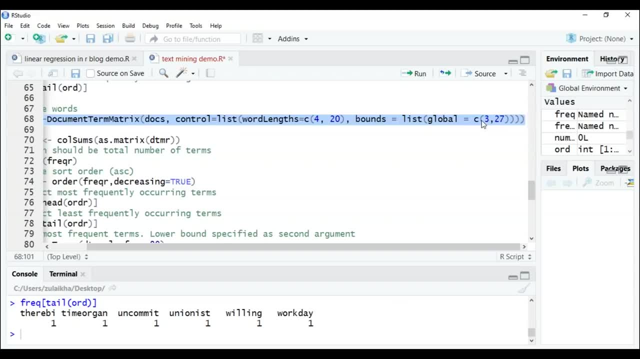 that text mining is an iterative process. okay, We have to keep doing these iterations again and again in order to clear our whole document. So I've given a bound over here of the frequencies of words that we should remove, So let's run that. 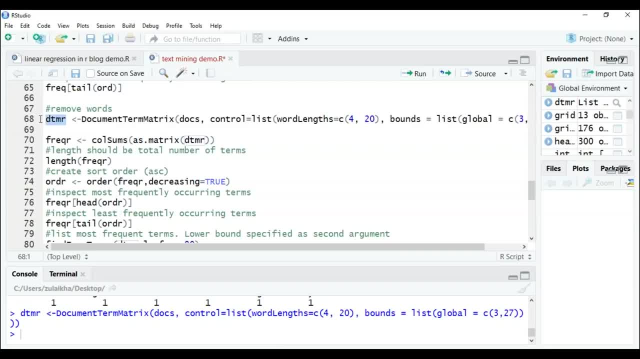 So all of these new words are now stored in a new DTM matrix called the DTMR. okay, Now I'm gonna just calculate the frequency over here, like we did earlier, and now we can also check the length. Okay, Now, this length is less when compared. 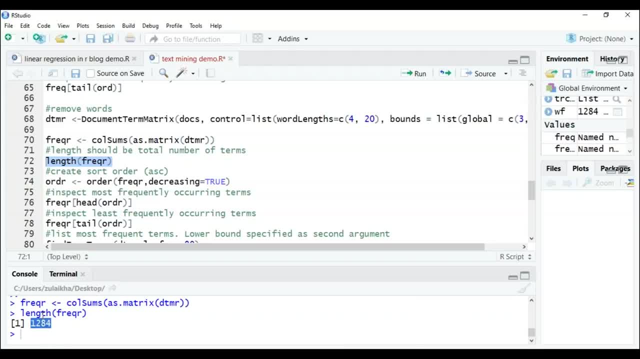 to the earlier DTM matrix that we had created. okay, That was around 3,000-something, and this is around 1,284 words. Okay, so what we're doing here is we're removing unnecessary words, okay, Words that are not needed or that are not important. 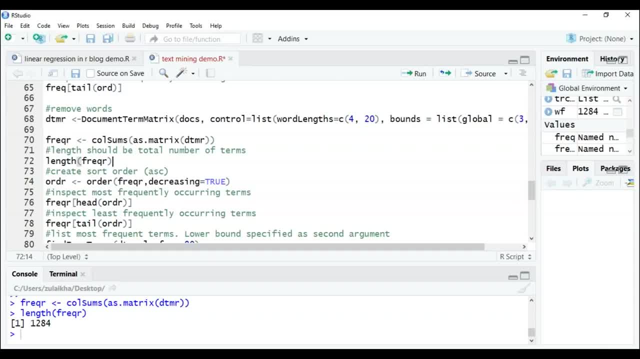 in order to understand the document. all right. So, guys, this is an important practice, because when you remove these words, you can finally focus on the important part of the document. all right, Now you can again create a frequency order list. 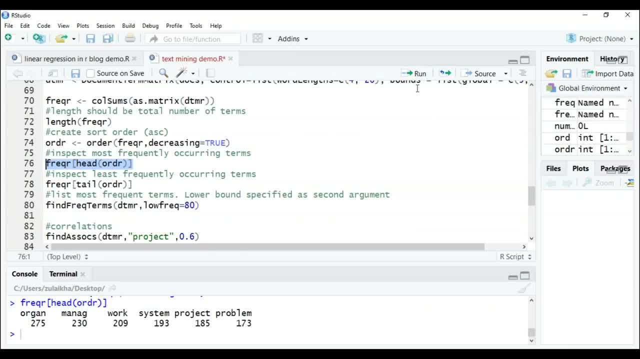 You can check the head of the frequency, all right. So this time the most frequent word is organ and there's manage, which has been cut down. there's work, there's system, there's project, there's problem. 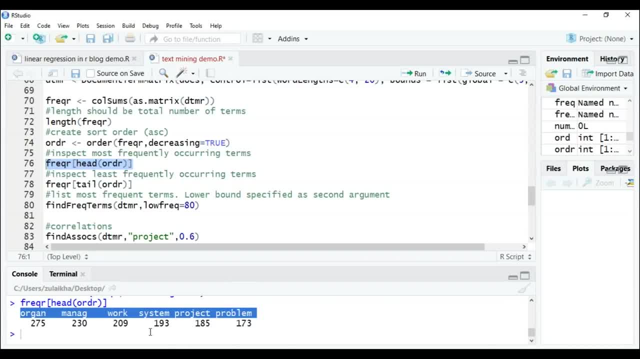 Now these words actually make sense. If we read this, we know that this is some sort of a business document or it's some sort of management or project document. okay, These words make sense. Similarly, you can inspect the least frequent words as well. 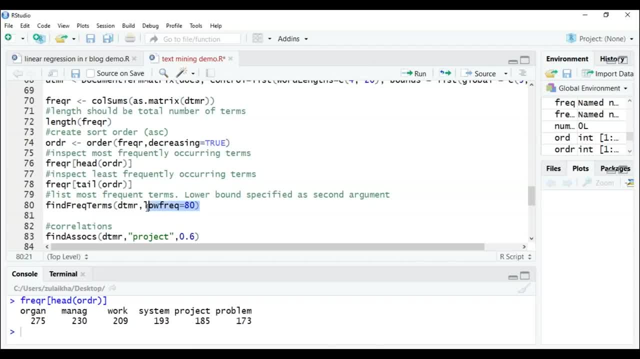 all right. Now what I'm gonna do is I'm giving a lower frequency bound over here. okay, I'm setting it to 80.. Now what I mean here is I want you to find all the terms or all the words in my document. 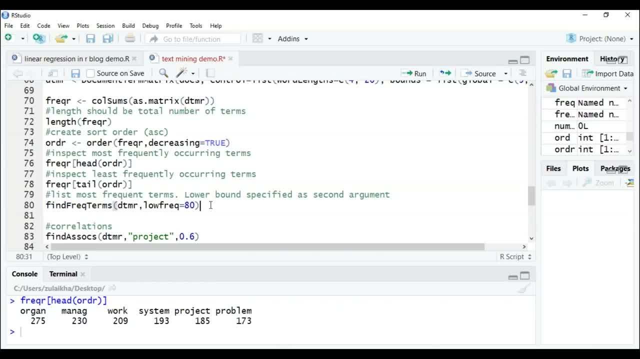 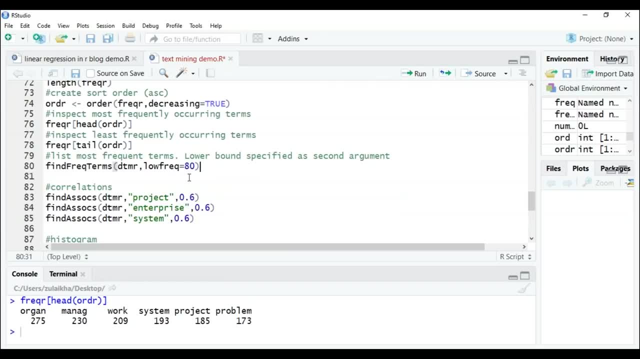 which have occurred at least more than 80 times. all right, Then, what I'm gonna do is I'm gonna find correlation between these words, because I know these words are important. They've occurred so many times in my document, meaning that my document is about these words. okay. 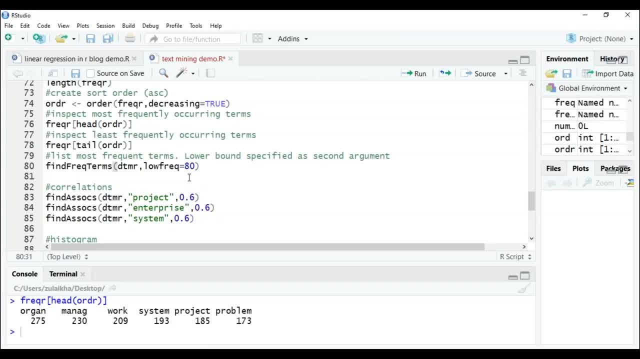 So once I get a list of the words that are most frequently occurring in my document, I'm going to try and find an association or a correlation among these words. Okay, so let's run this code and let's look at our most frequently occurring words. all right, 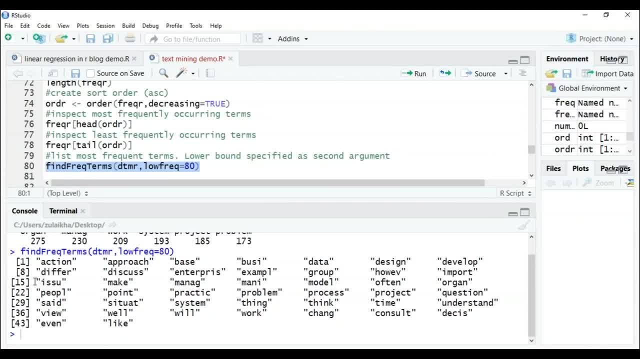 Now, thankfully, we don't have a lot of stop words over here, even though I do see a few words which are not needed, like, for example, said like and all of that- but there are some essential words, like data. 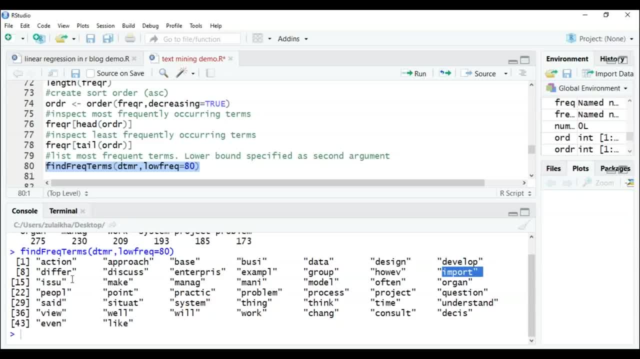 there's design, there's develop, there's import. okay, All of these seem important to me, okay. So, guys, like I mentioned earlier, it's an iterative right, It's a process. You have to keep performing text analysis. 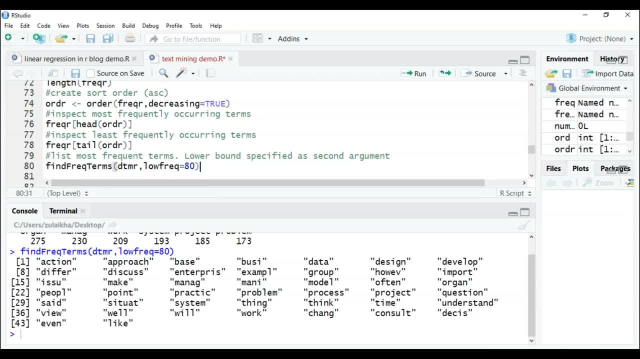 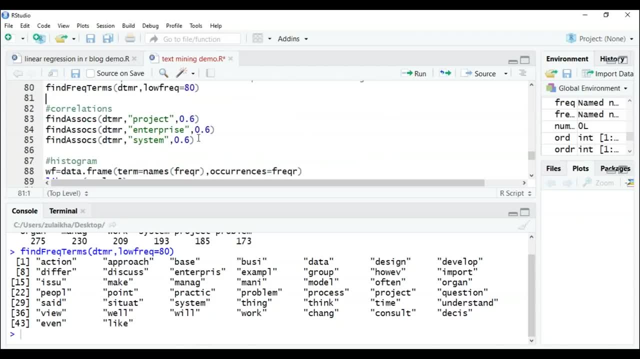 over and over again. So, guys, you can perform other approaches as well. okay, You can perform lemmatization Here. I showed you how stemming was done. all right, Now let's look at the correlations. okay. 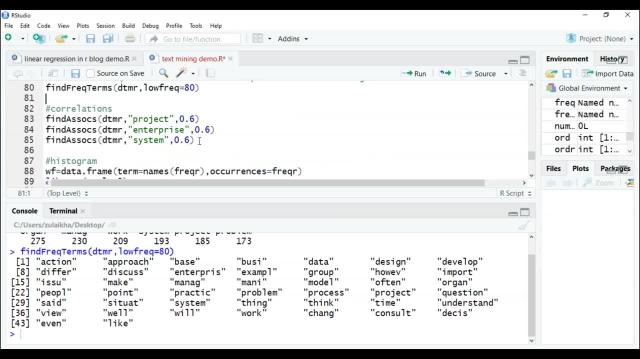 We're gonna try and find the correlations between specific words. Now, when I say correlation, I basically mean it is the co-occurrence of words in a multiple document. okay, so which two words occur more often? That's what I'm gonna check, okay. 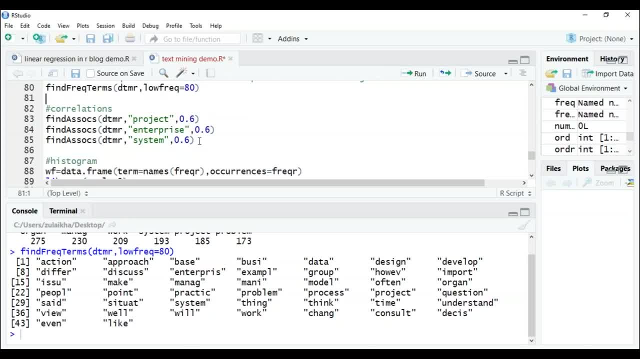 I know two words are occurring oftenly together. I know that they have an association or a connection between them. okay, Now the TM package, or the text mining package that we installed at the beginning. it provides a function known as findAssociation. 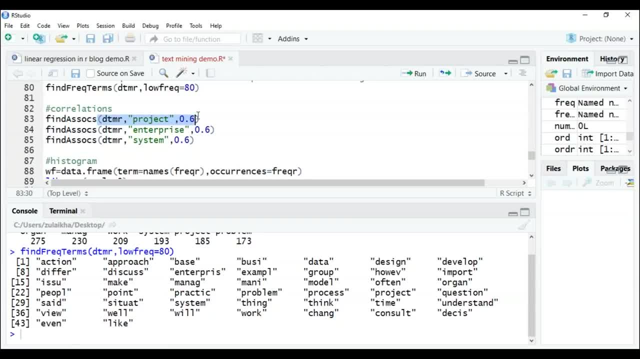 okay, this function. Now, this function takes in three parameters, like you can see. okay, The first parameter is your DTM matrix, your document term matrix. The second one is the term of interest- okay, the term that you want to find association with. 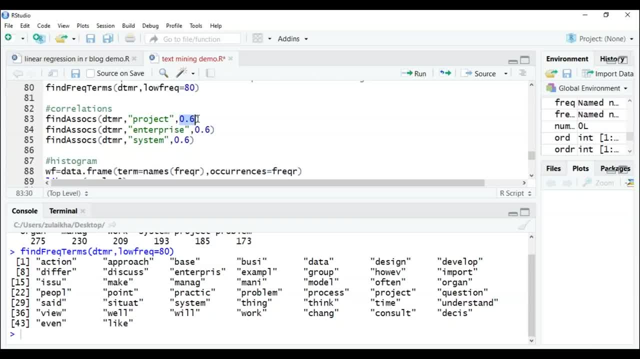 And the third one is: so this is basically the correlation limit. all right, all right. So here we've chosen three words. We have project, enterprise and system. What we're gonna do is so here we're gonna find: 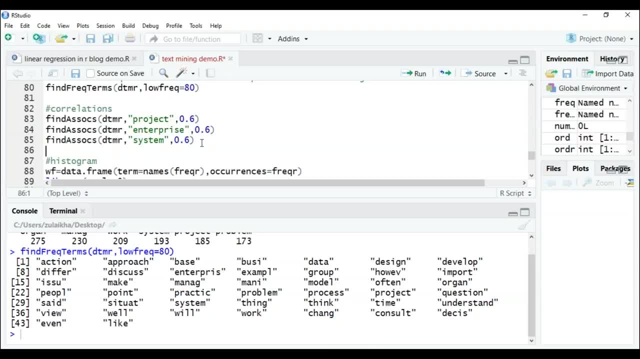 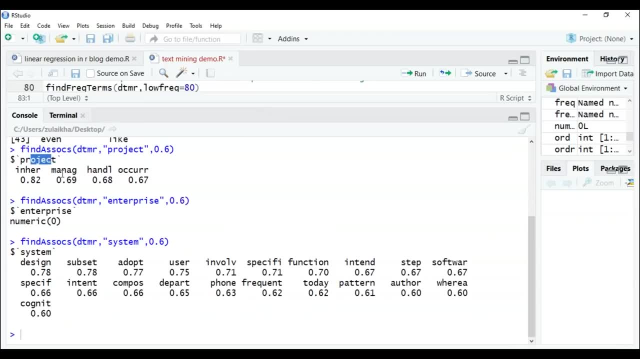 a correlation of at least 60%. okay, Let me run this and then you'll understand what I'm saying. all right, Okay, so basically, project and inherit and project and manager, project and handle and project and occur, Occur- these many times together. 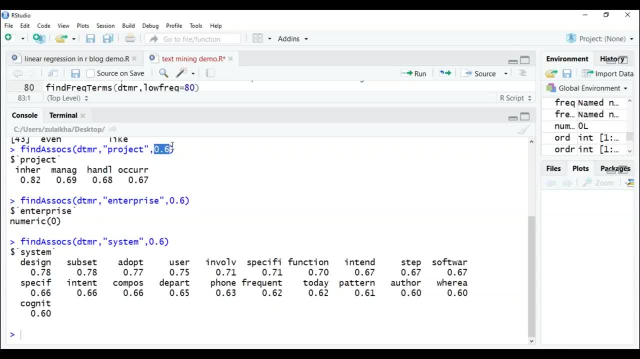 Okay, this is a correlation, So basically about 0.6 or about 60% correlation. I'm checking how many terms occur with project, Similarly with enterprise. I've not actually got anything for enterprise, meaning that there's no other word. 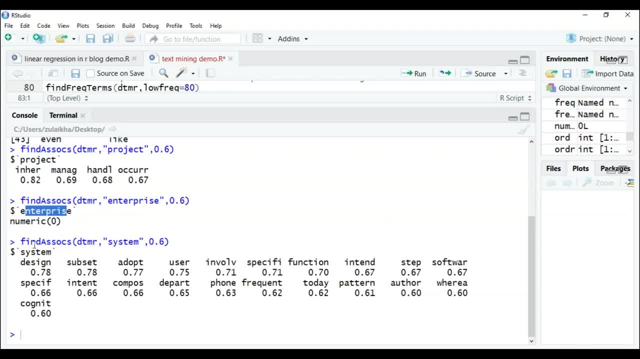 which co-occurs more than 60% of the time with enterprise. Okay, now, when you come to system, you can see that design occurs, subset occurs, adopt occurs. Now, this is an interesting combination. okay, It'll actually give us a lot of insight. 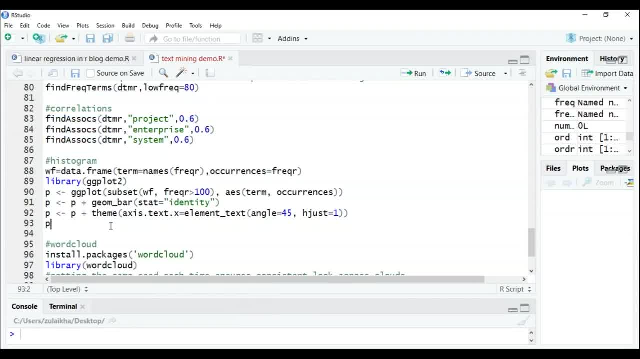 about what the data is talking about. all right Now, once we're done with that, we can finally move on to our graphical analysis. okay Now, one of the really cool things about R is its graphical capability. okay, So first we're gonna do a simple frequency histogram. 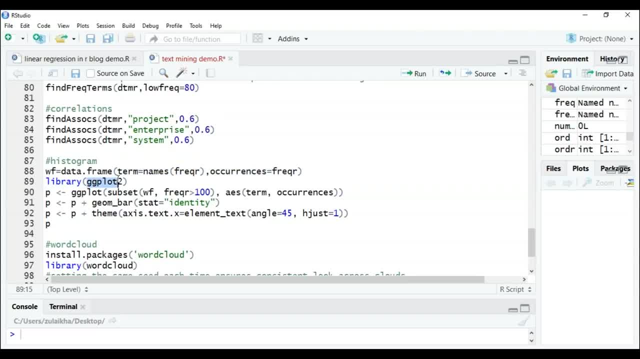 Here, I'll be using the ggplot2,. all right, I'll be using this package and this is the entire code. Now, first of all, we're just creating a simple data frame. all right, it is a list of columns of equal length. 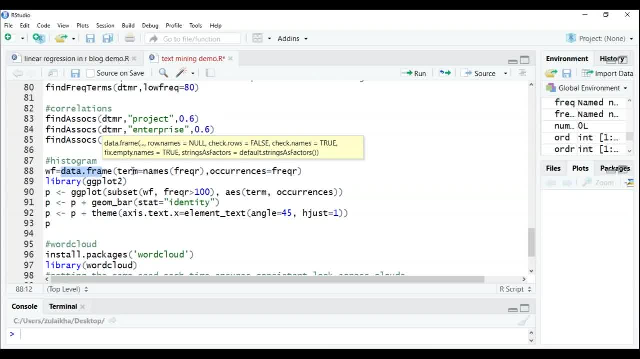 After that, we're saying that the data is. the data frame also contains the name of the columns and in this case, these are the terms. These are basically the terms and the occurrence, respectively as frequencies. all right, So let's run this entire code. 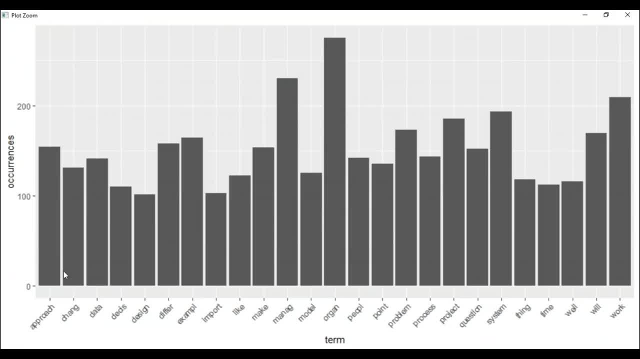 and let's look at our histogram. all right, So if you see that the most frequently occurring term is organ, okay, We have manage as well. okay, We have project, we have system, we have thing approach. Now, this is basically used to give you. 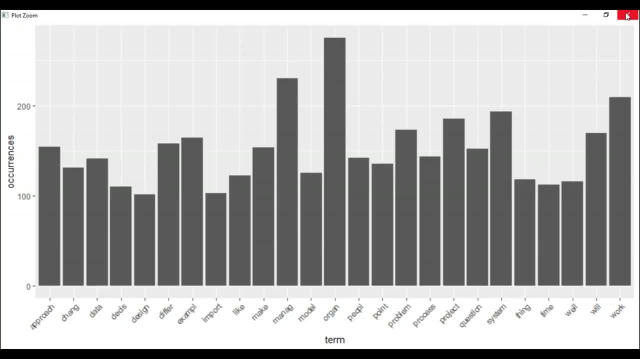 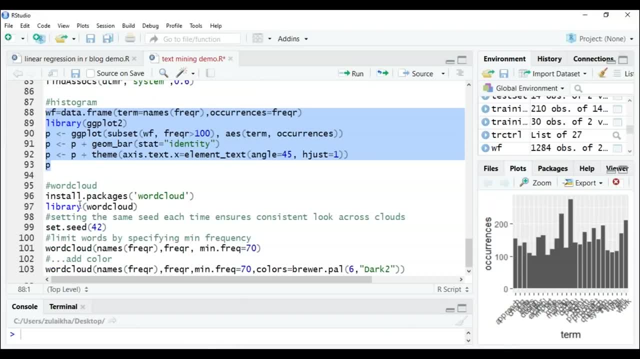 a graphical analysis of which term or which word occurs more frequently. all right, So, guys, this is a simple histogram, and we use the ggplot2 library for this. Now let's create a word cloud, because everybody is doing this on the internet. all right? 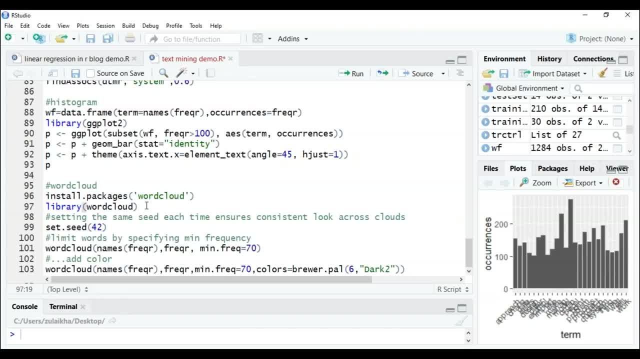 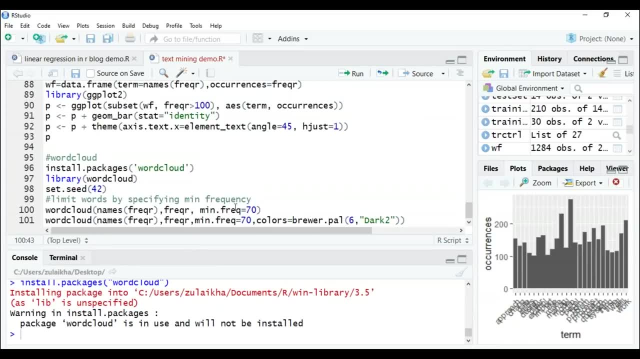 So first we start off by installing the word cloud package and by loading that into our studio. okay, So let's run this. All right, you can specify the frequency of the words that you want to be plotted over here. Okay, here I've limited it to 70,. 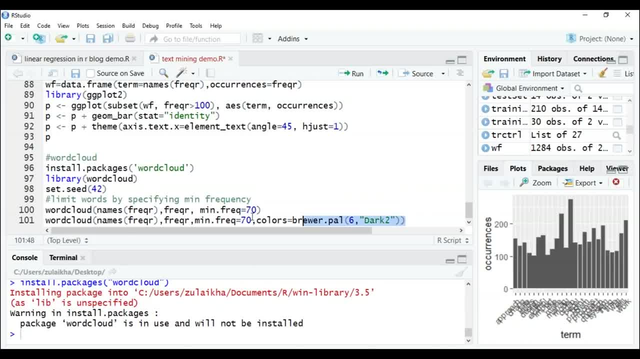 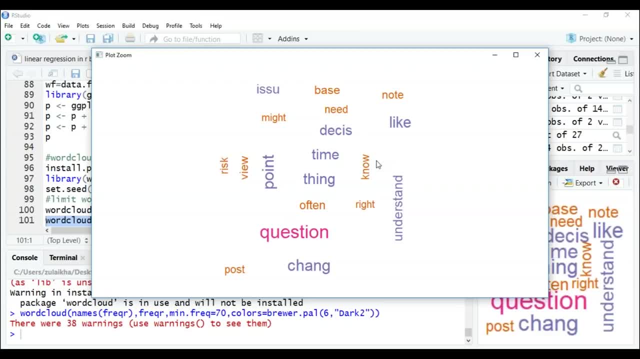 but you can increase the frequency or decrease, depending on your choice. all right, Let's run the word cloud and let's see how it looks okay. So if you notice the word cloud, you can see that the stop word removal was not done correctly. okay, 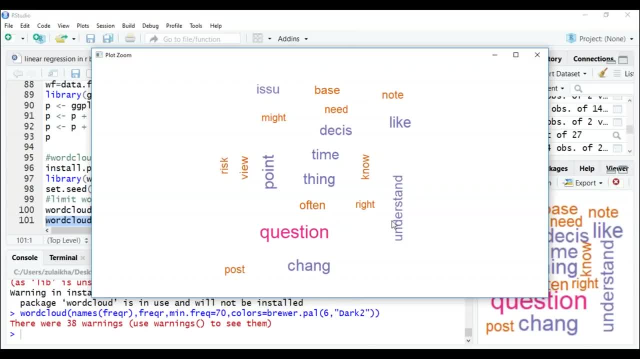 Because there are a few words I can see over here, like know, often write and like. All of these are not important words, okay, They are stop words. So what you can do to avoid such mistakes is you can create a custom list. 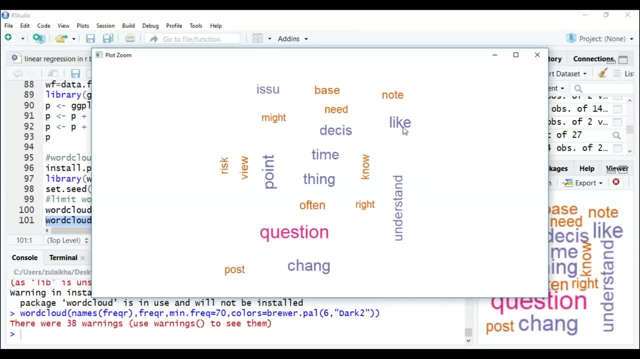 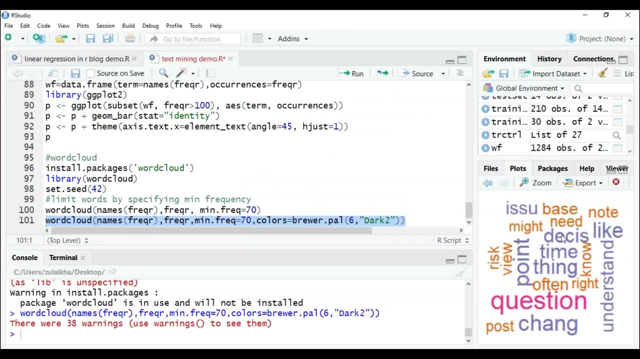 of all the stop words. okay, You can create that, and then you can run an R code that will remove all the stop words, okay. So, guys, this was our entire demo. So, guys, I'd like to end the demo by telling you all: 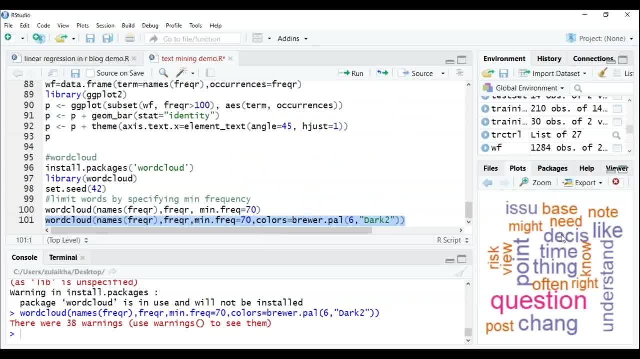 that text mining is an iterative process, okay, So you can't get everything right at once. You'll have to form a lot of cleaning, like we saw in the demo. We need much more cleaning in the demo. I'm going to leave that up to you guys.